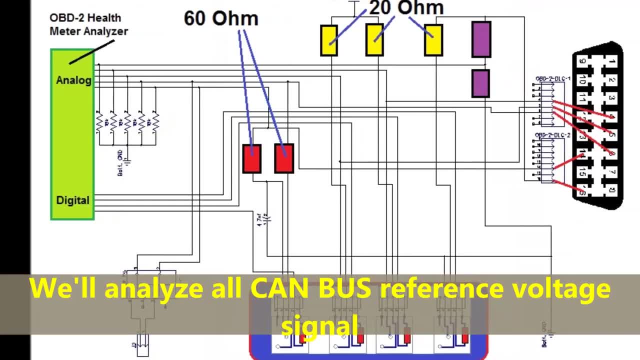 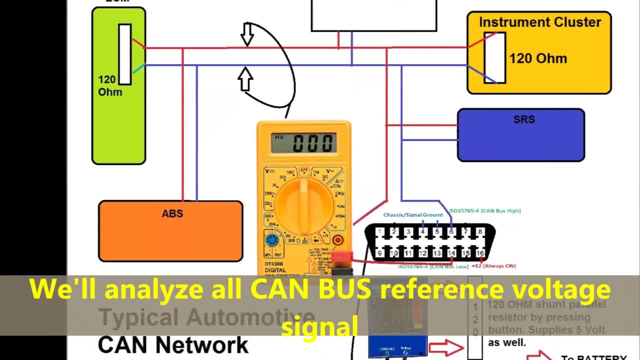 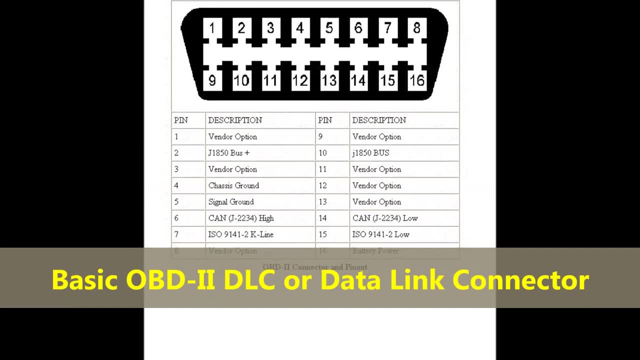 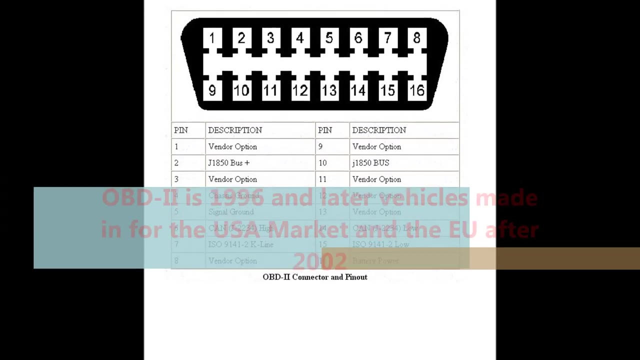 And we're also going to explain how, the voltage that you see at any CAN vehicle, how you arrive at these voltages And there's a lot behind it. so, anyhow, bear with us. But first a few basics. This is a basic OBD2 DLC, a data link connector, on any automobile made after 1996.. 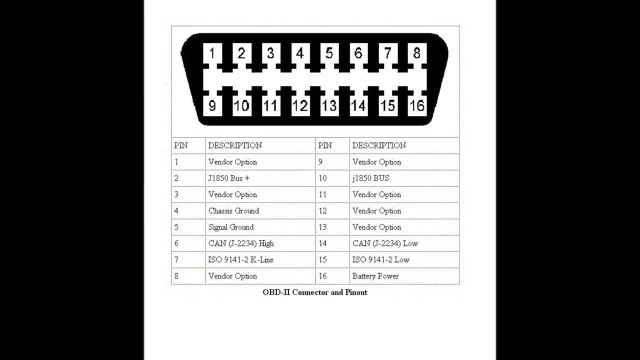 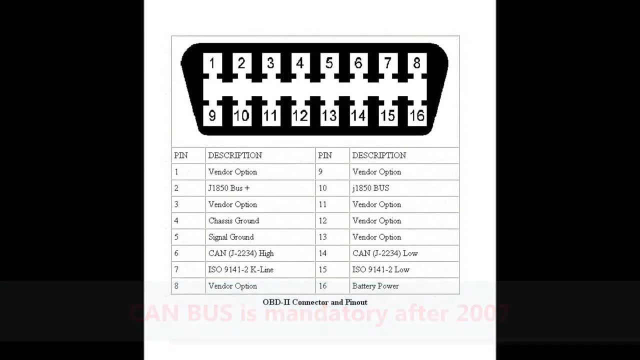 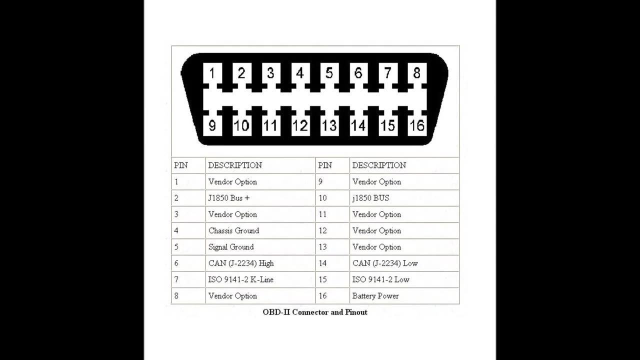 In this particular case, almost everything nowadays. after 9th, everything became CAN Controller Area Network, which was developed originally by Bosch. Now pin number 6 and 14 are the ones that are going to carry the signal. Now these are the pins mandated by law. They all have to have pin number 6 and 14 running CAN. 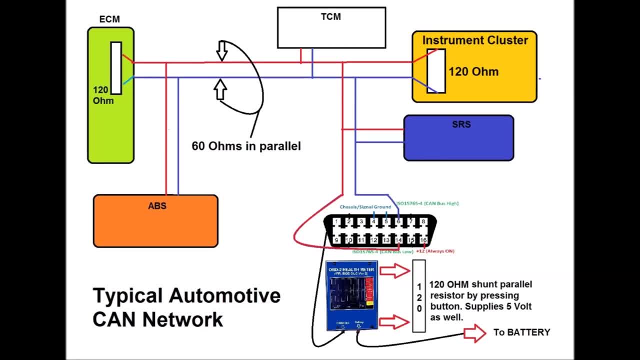 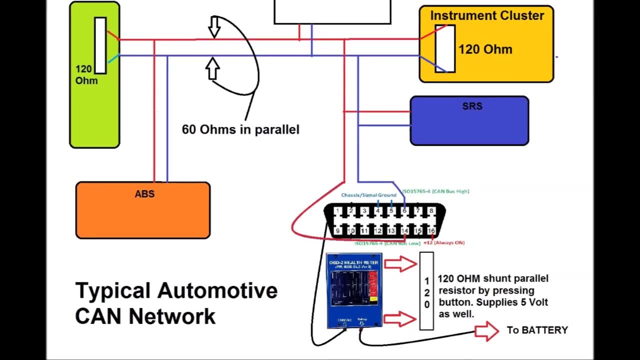 They may. for example, there's a slow CAN and there's different variations of CAN that run on pins number 1,, for example, and this, this, and that We're not going to talk about that. We're just going to concentrate on CAN vehicles Controller Area Network as it is mandated by OBD2.. 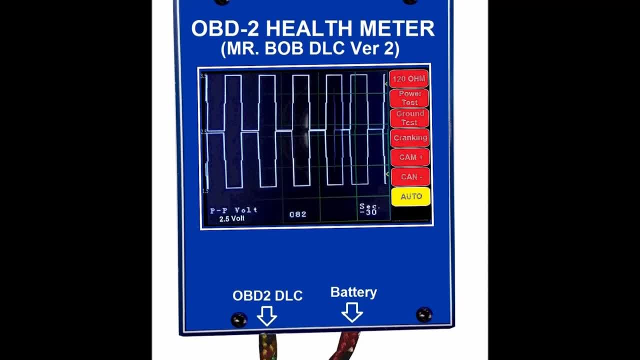 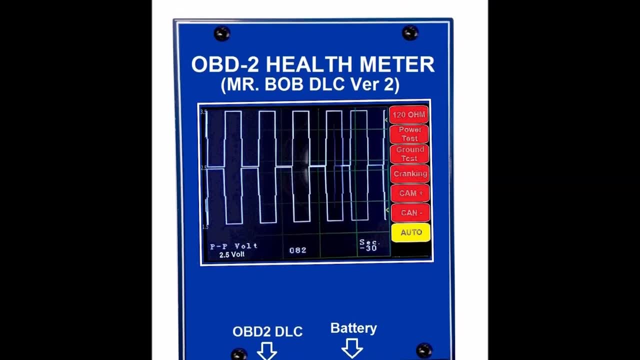 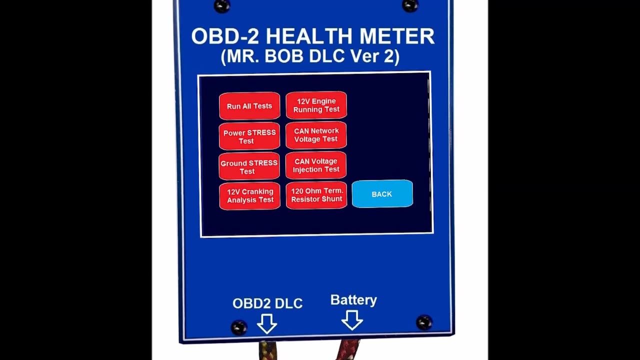 As you've been seeing on screen, this is the OBD2 health meter. It is a dedicated unit that we actually manufactured and designed and developed, which just introduces into the market, So it's very handy when it comes to OBD2 diagnostics, running, testing, power and grounds and so on and so forth. 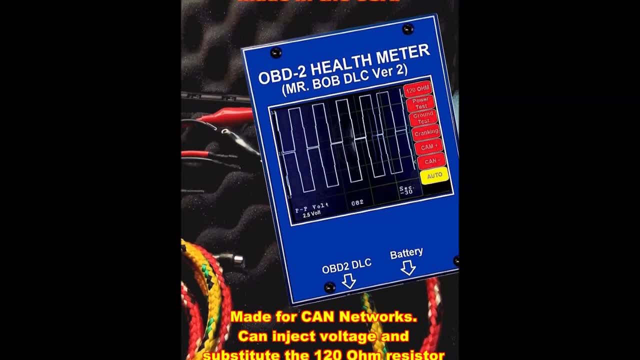 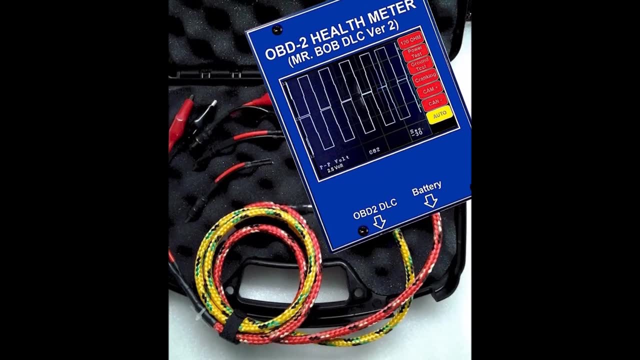 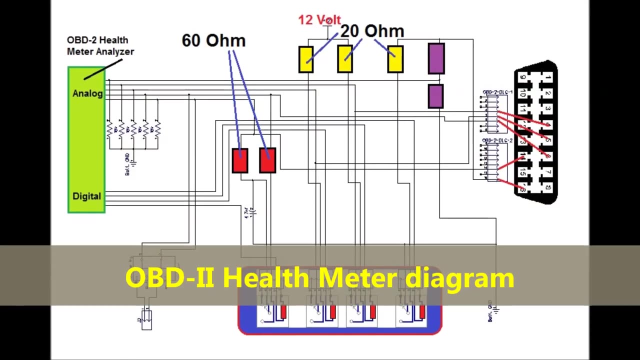 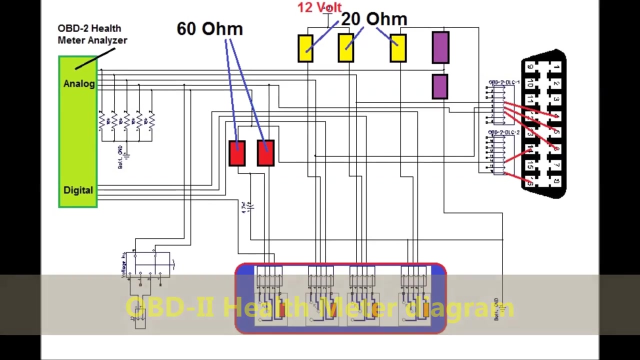 The video is not necessarily about this unit, but it's just. you know, basically we some of the stuff that you see on this video were actually captured or enforced: The OPD2 Health Meter. Very quickly, as you can see on screen this unit, it's loaded with a bunch of electronics inside that actually stress the power: the DLC power, the chassis ground, the sensor ground, the pin number 16 power. 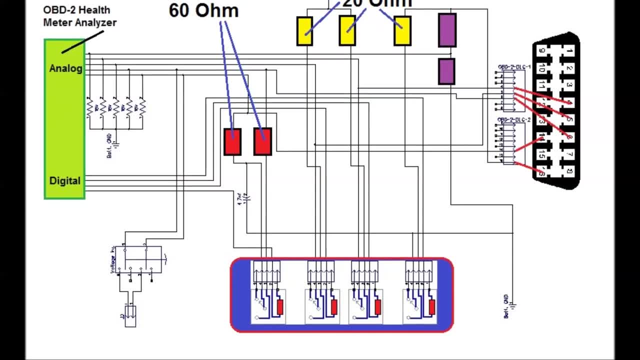 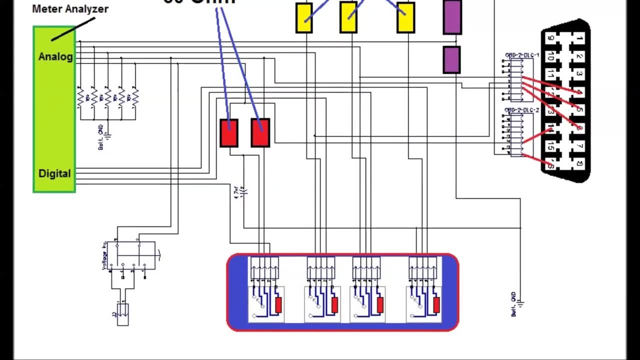 Oftentimes you have issues with that and the sensors and the grounds, and you really don't know unless you actually test them, And they're causing all kinds of problems And they're causing all kinds of problems. And they're causing all kinds of problems. 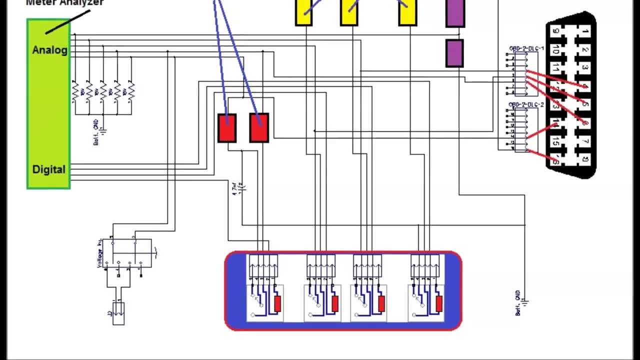 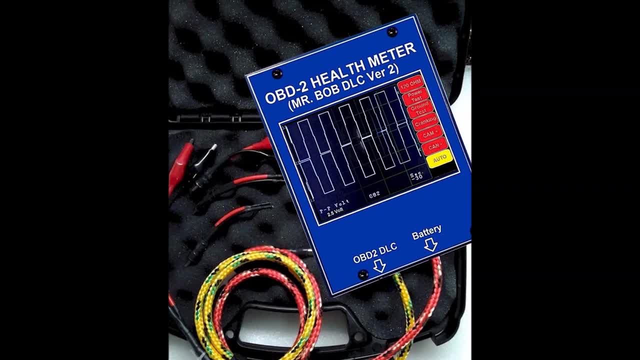 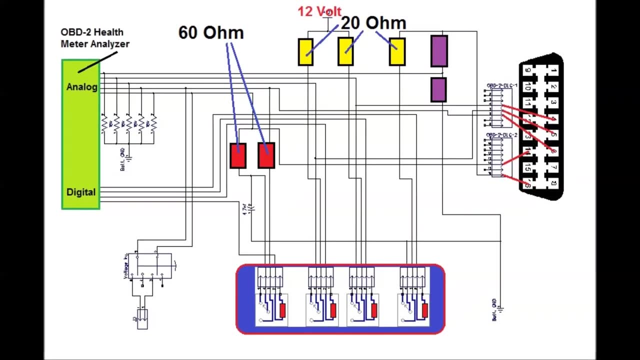 of problems on your uh, on your uh readings, uh, uh for the, for the scanner, and it's not. there's nothing wrong with anything, it's just that you have a, a faulty ground or power. so the unit has these big resistors on top, as you see on screen, um, in yellow, uh, there are 20 ohm resistors. 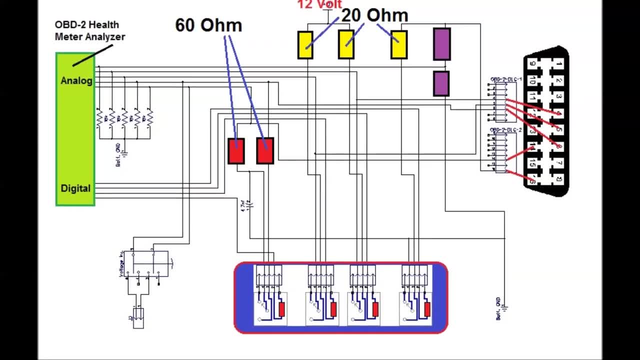 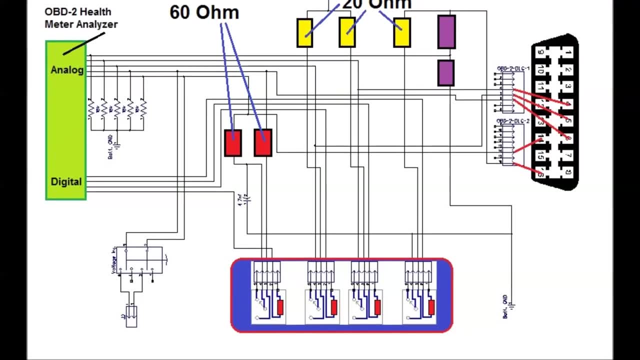 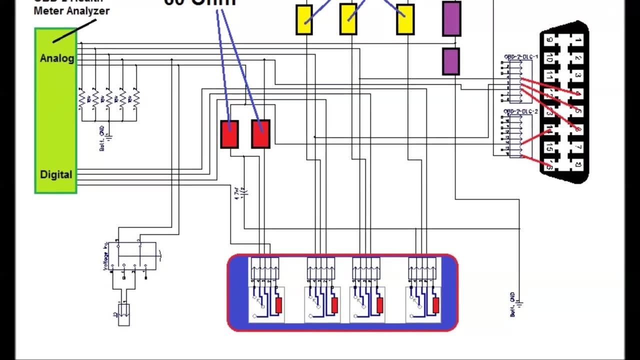 that the unit actually shorts the ground and the power and it actually measures. you know, there's a computer inside that actually measures and there's a screen, as you saw, uh, as you actually can see on screen right now, um, anyhow, and there's, uh, there's also other stuff in there too. you can. 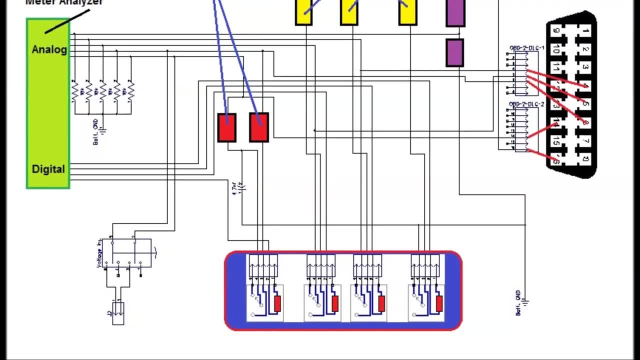 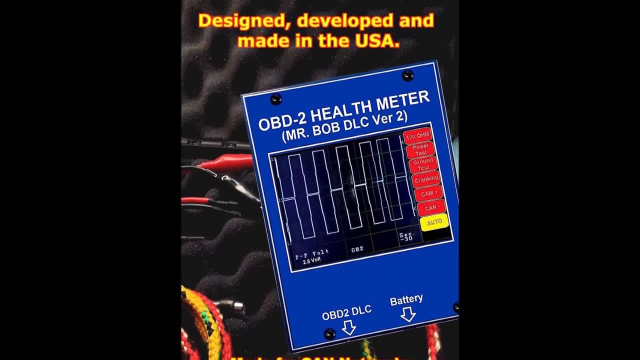 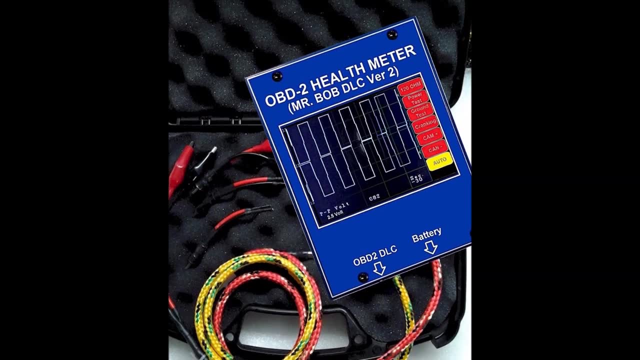 actually substitute the 60 ohm termination resistors with this unit. uh, it actually injects a voltage also on the can uh signal. in case you're missing it. uh, there's a bunch of stuff, you know that, that you can actually do with this unit, uh, and that it actually, if you need to, 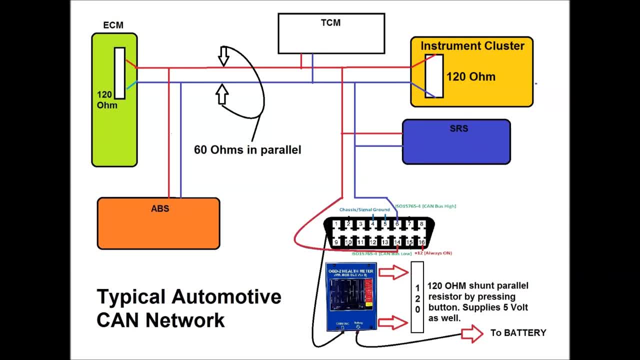 understand about camera. you need to understand about camera. you need to understand about camera vehicles and how it is structured, and that we're going to talk about that here. as you can see on screen, this is what a a can network uh has to. uh has to look like they're, all the same, the only. 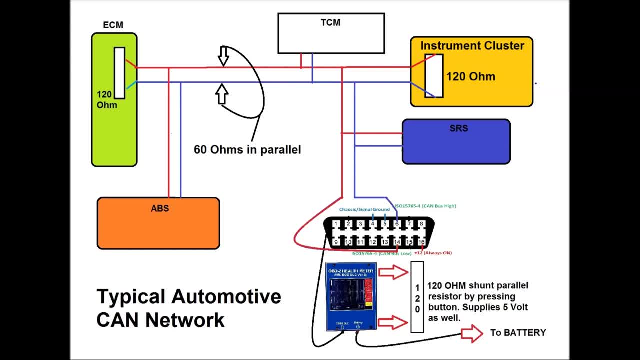 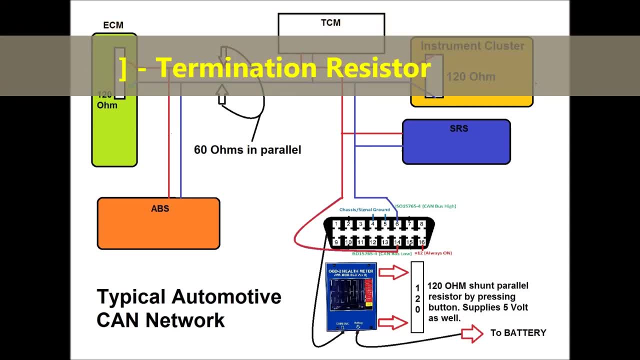 thing that that changes is the amount of modules and this is a simple can where you see the instrument cluster, the transmission control module, the acm um uh. there's also the uh abs module in there and, as you can see, the instrument cluster, the transmission control module, the acm um uh. there's also the uh abs uh module in there and it's 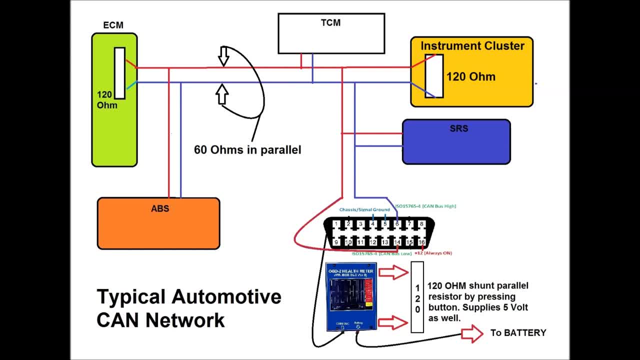 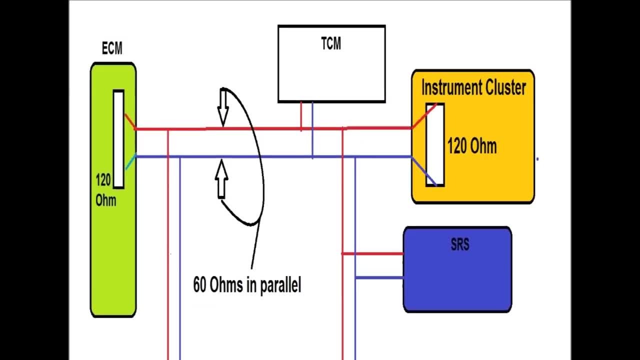 you can see the instrument cluster, the CCM module, the sdm module and, as you can see, you have, you have to have two termination resistors. so this is, this is basic when it comes to uh, to cat networks, uh between the two termination resistors, if you, if you have two resistors in parallel, as you see on. 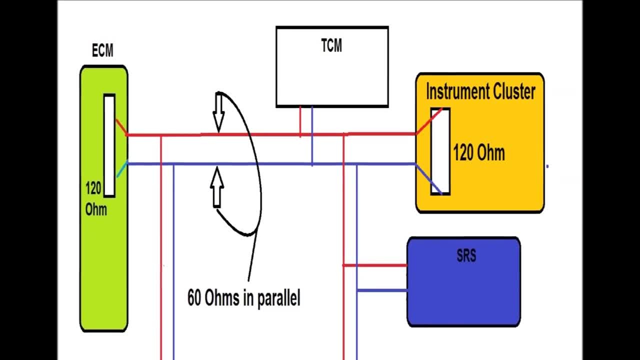 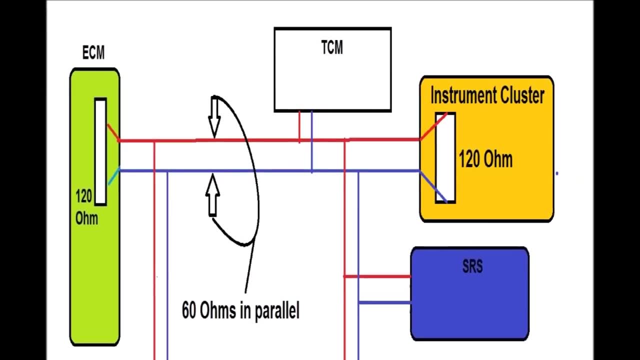 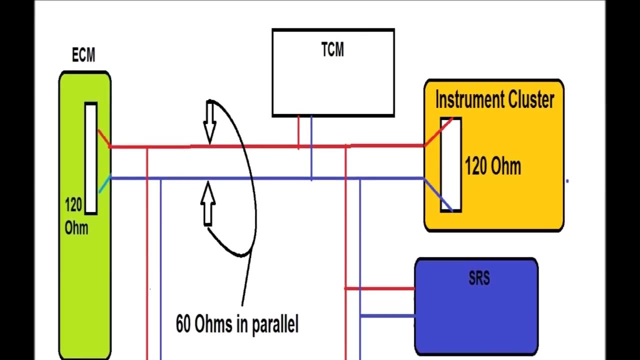 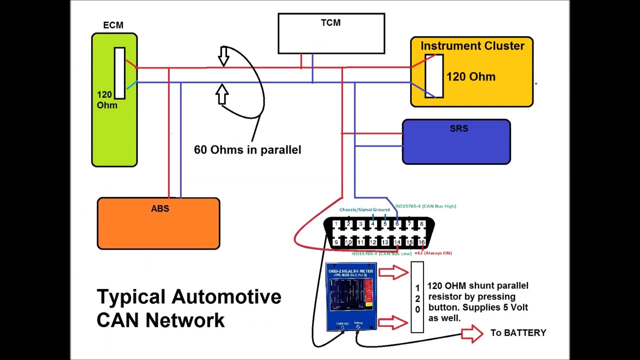 screen. on this diagram you're going to have 60 ohms. if you measure the uh, the two pins, pins number six and fourteen, you're gonna have sixty ohms and that's exactly. give or take a couple of ohms, usually 60, 62, 63, 58, something like that. doesn't have to be exact but close. so basically, 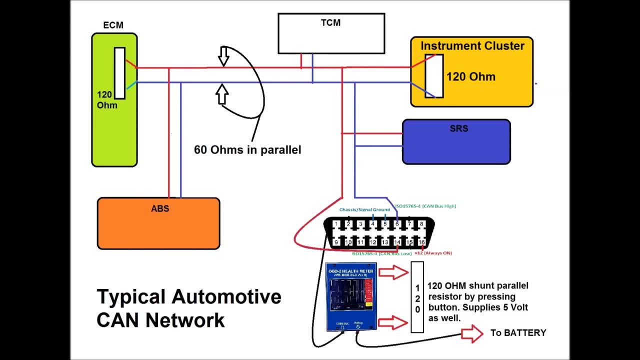 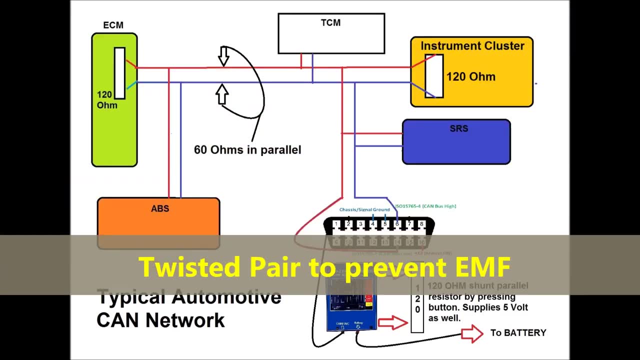 you're going to. once you have two 120 ohm resistors in parallel, you're going to have 60 ohms across both wires. you know, on the can and these are usually twisted pair wires. they're twisted and this is to prevent emf electromagnetic interference. now it is important that these 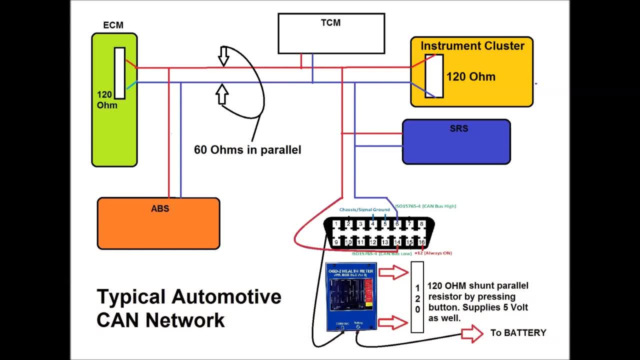 120 ohm resistors. you may lose one of them and, depending on the vehicle, it may or may not operate. uh, but you need to find where these- and this is usually the instrument cluster- is. the one is one of them that almost always has the one. one of the 120 ohm termination resistors, the acm. 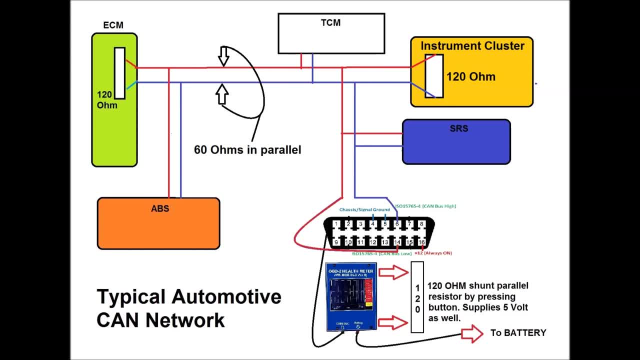 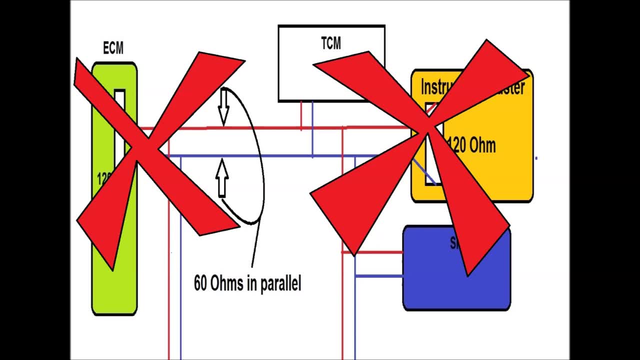 acm, acm. acm normally carries the other 120 ohm resistor. now, if you lose these resistors, often times you have no communication. and if you measure across these two wires, basically pins number 6 and 14, you're not gonna see 60 ohms, you're gonna see. 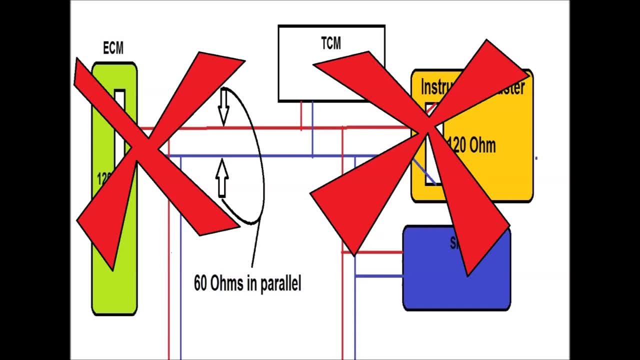 you might see 120 ohms, or you might see infinite. that means you lost both resistors. or you may see zero. that means you're shorted, that means the CAN network is shorted, the two wires are shorted. then you're not going to have communication. 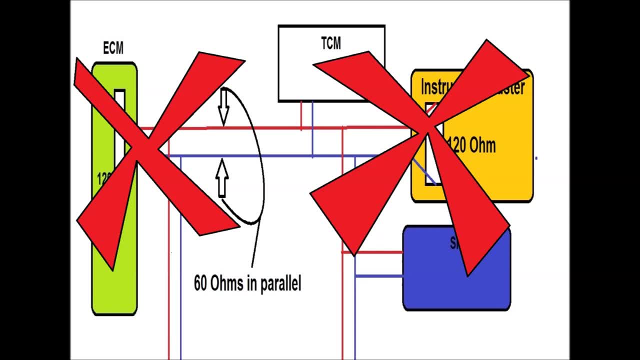 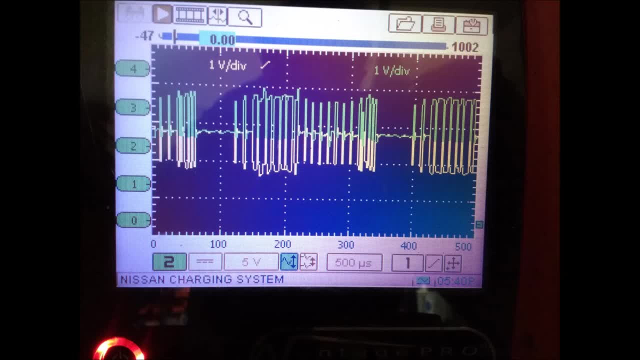 in our video. here we're going to initiate communication, we're going to show you what it looks like on an oscilloscope, and this is probably the best way to do it now. but before we go into that, basically the unit as you can see on this particular diagram. 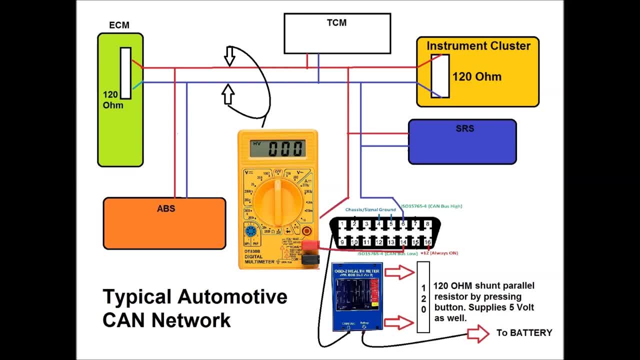 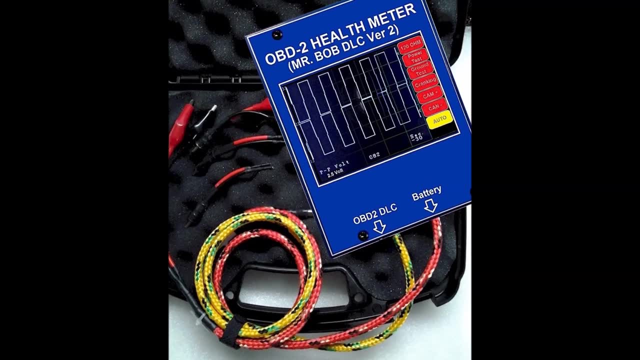 the OBD2 connector has gives you access. this is the easiest way to give you access to these two pins. pins number 6 and 14: okay, our unit, the OBD2-DLC health meter, actually goes in there and plugs into power and ground on. pins number 16. 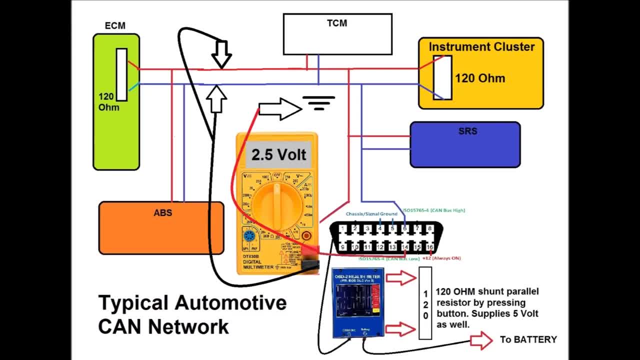 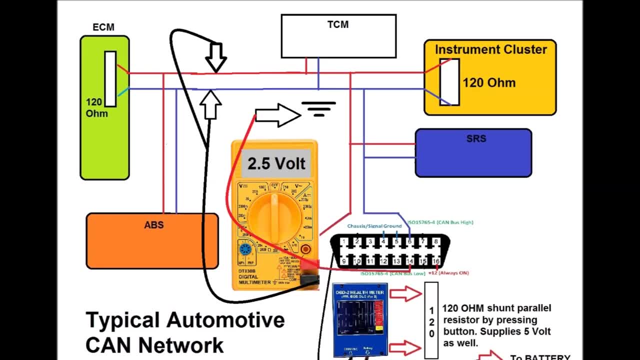 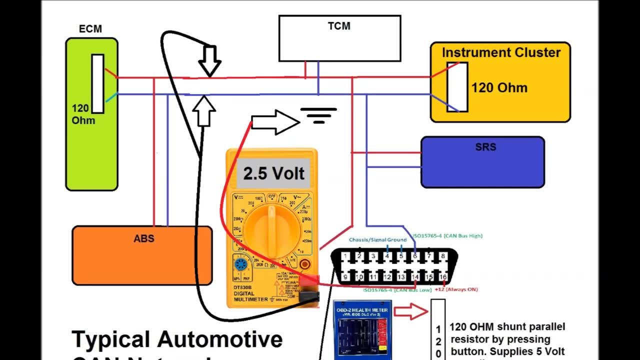 which is power 4, 5 and that's it. that's how you power the unit on a 4, 6 and 14 for the CAN network. the unit then substitutes a bunch of depending on the tests that you actually pick on your on screen. it's got the has a little screen touch screen in. 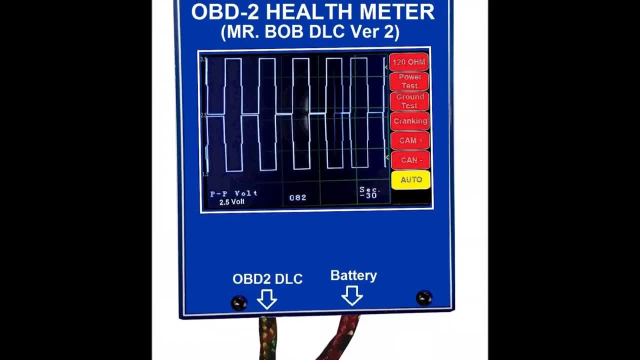 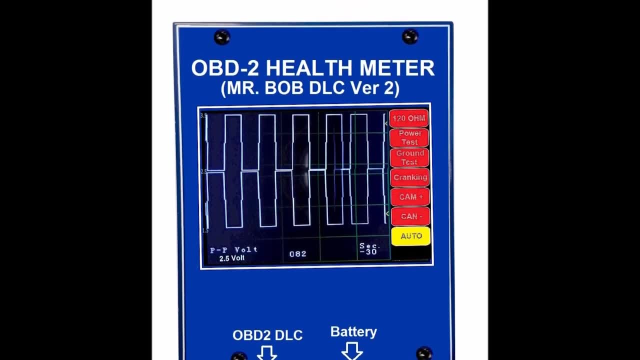 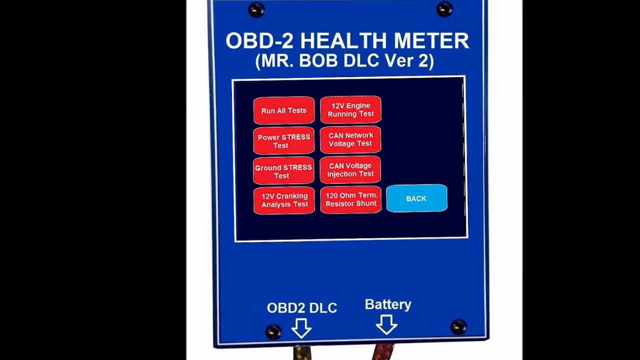 there and you actually choose either the automated test and it actually runs the all the testing in there, or you can actually pick and choose which test you actually want. it has a like an oscilloscope, but it's not an oscilloscope, it's more of a graphing multimeter. 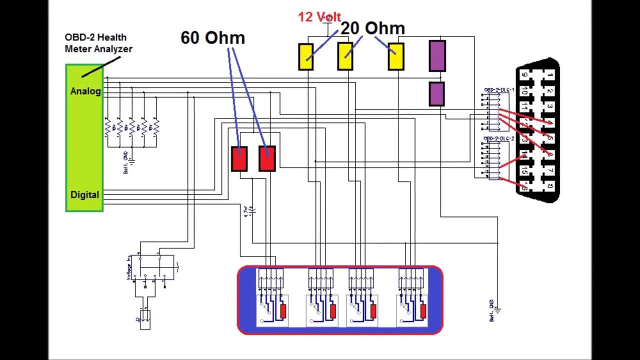 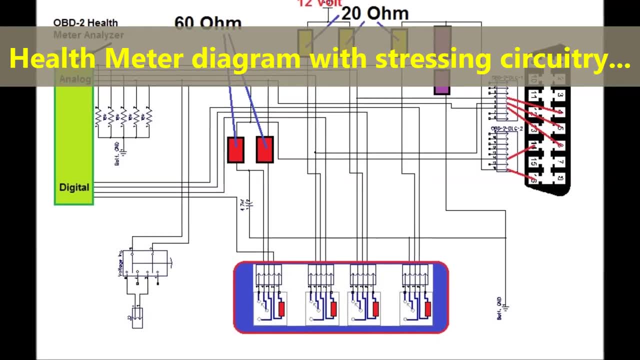 where you can actually see what we're going to see now. we're going to see that later on. in this video you can actually see the, the signals and you'll know right away, and the unit is also going to analyze the signal for you. this is what's different about this unit than anything else that you you can plug in anything you. 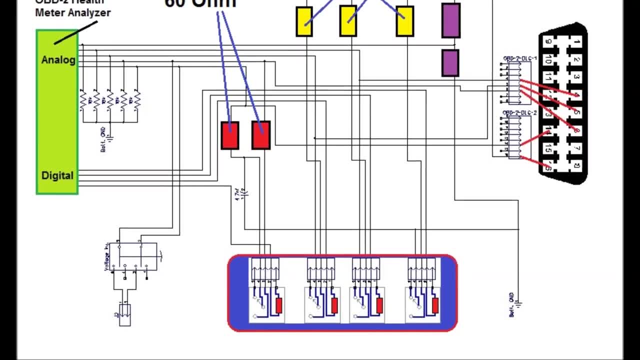 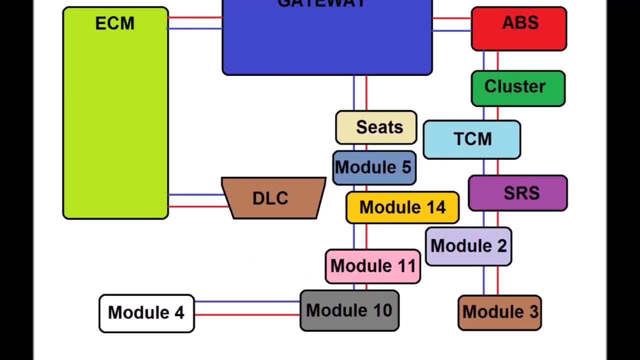 want like an oscilloscope, and this and that, and if you don't know exactly what to look for, which we're going to show you here anyways, but some of you may not really be into it, you know, and you still have a car with no communication. so what are you going to do? 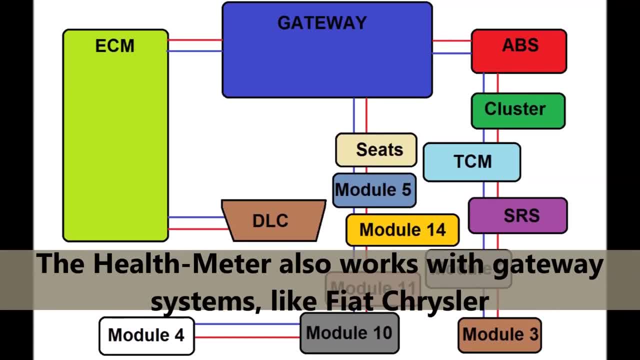 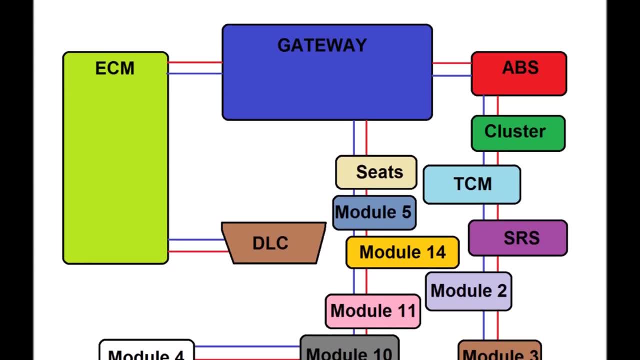 so this unit, it's automated and it goes into a bunch of tests that you don't even know that it's doing it and it's pretty much you know. it'll tell you, you know. if you have an issue now on screen, let's start by analyzing this signal that you're going to see, either on the unit, on. 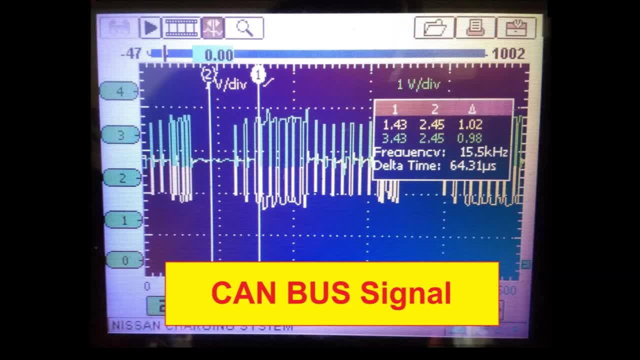 the obd2, obd2 dlc health meter, or on an oscilloscope. in this particular case, we are going to use an oscilloscope because the screen is bigger and we can actually show you in a better format basically what we did and you're going to see later on in the video you're going to. 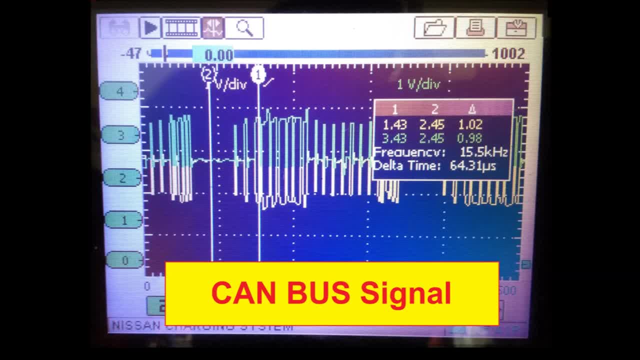 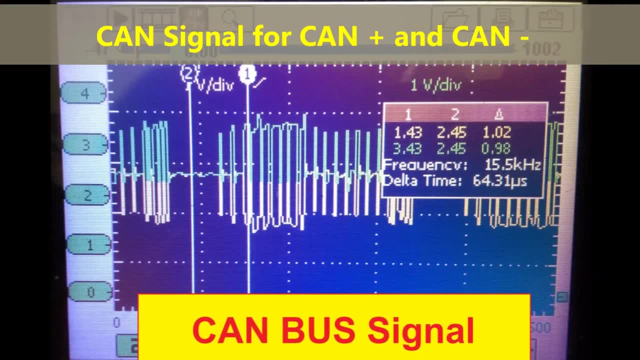 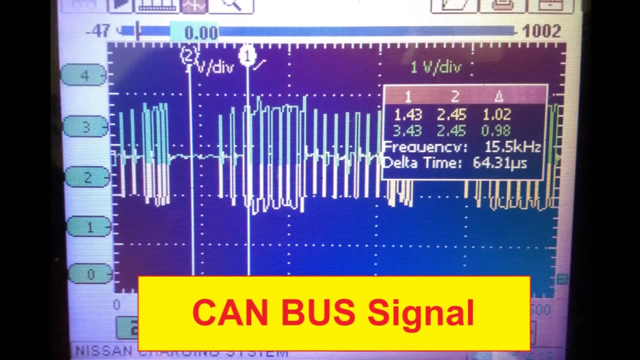 see that we actually made a virtual canned network. this is what we're doing right now, but, anyhow, what you see right now it's a? uh, this is the CAN signal for both wires. okay, the yellow one is for the CAN low and the green one is for the CAN. 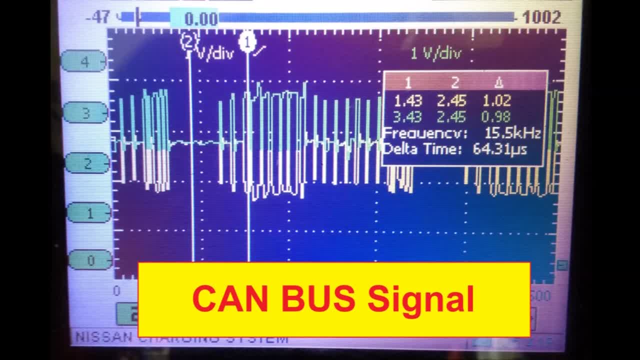 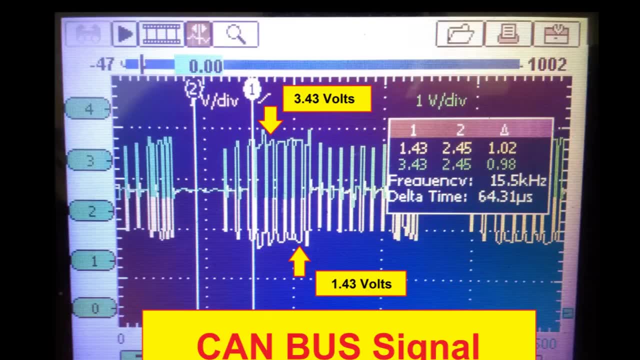 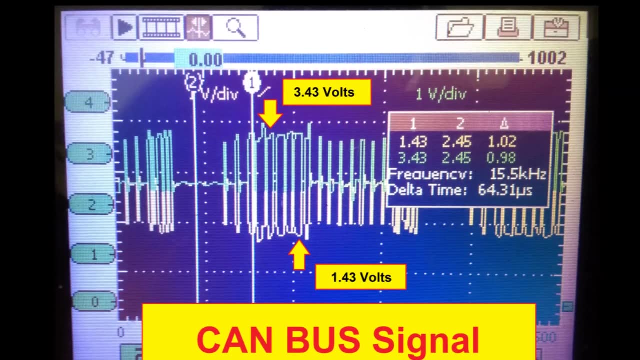 high. now very carefully. let's look at the screen as you see it right now. on this, on this particular diagram, if you were to measure with a, with an ohmmeter, uh, the resistance between the two uh wires- okay, not the resistance, I'm sorry, the uh, the voltage with the uh with the vehicle key on. 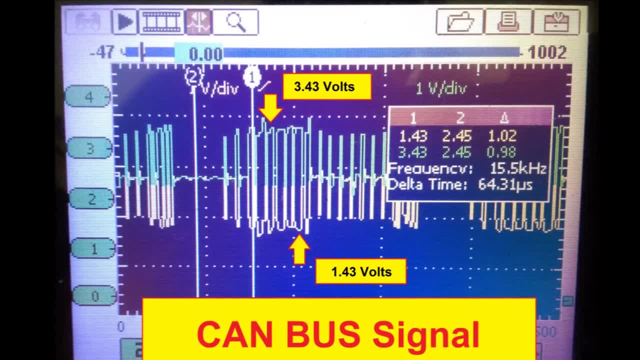 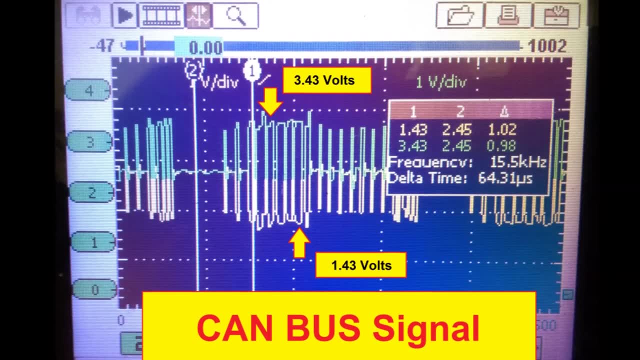 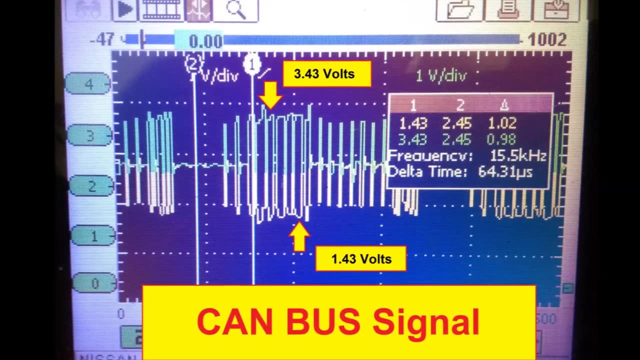 engine off. uh, basically what you would see between the two, uh CAN wires, CAN low and CAN high, pins number six and fourteen, you're going to see zero volts. okay, this is important because everybody gets confused when they see it. they say, well, I have zero volts, I have no, so I have no communication. 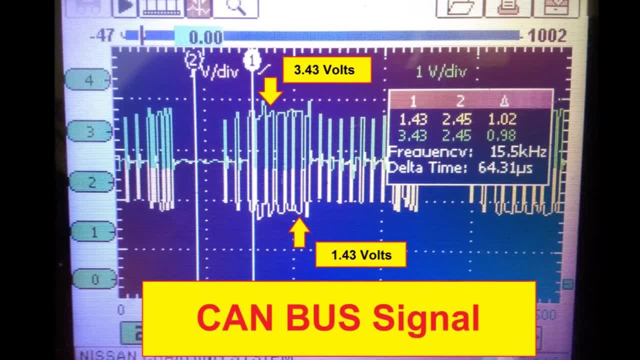 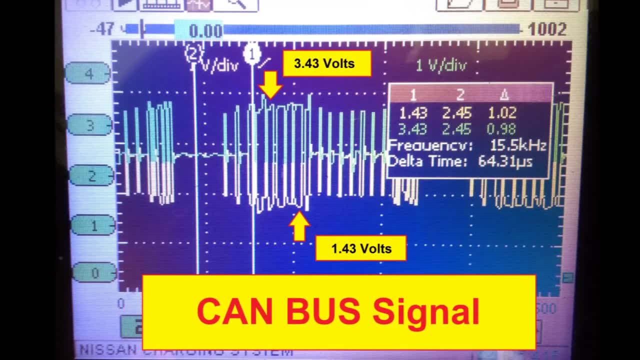 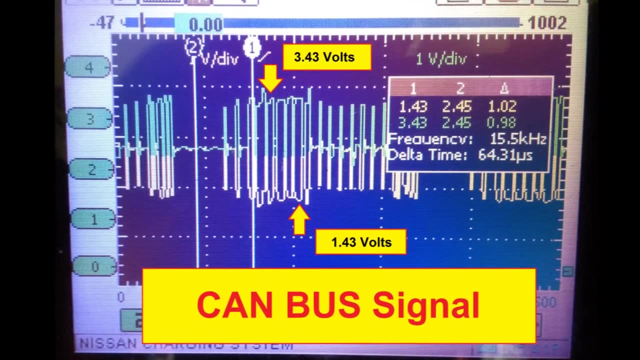 zero volts. something's wrong. no, you're. you're supposed to see zero volts in the? uh. in the old days, back in the 70s and 80s, uh, sometimes we used to install radios- car radios, uh- which had floating grounds, the speakers had floating grounds. there was no ground. the ground. 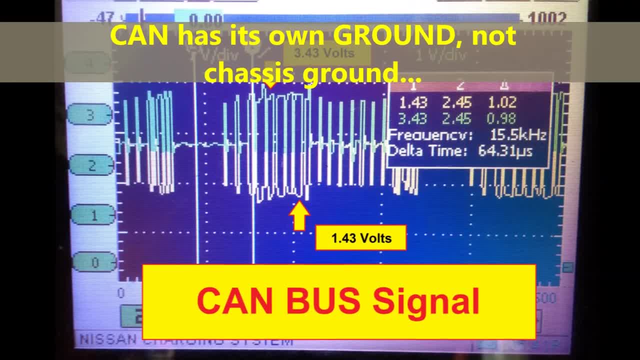 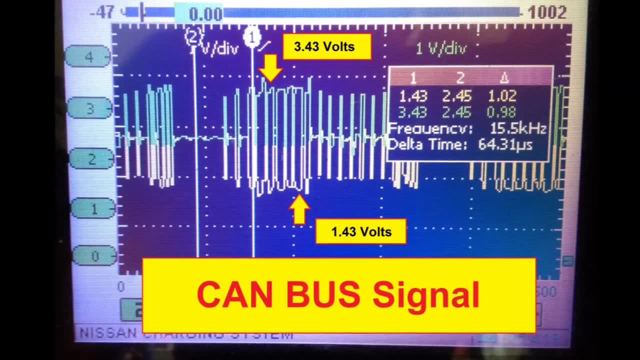 for the speakers was not the same as the vehicle ground, and so they were, you know, finicky. you know back then people would not understand that and so basically, this is what it is. uh, a CAN system has a floating ground, so the ground has nothing to do with the uh, with the battery. 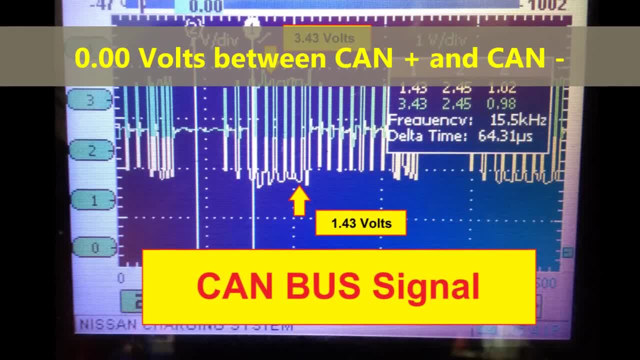 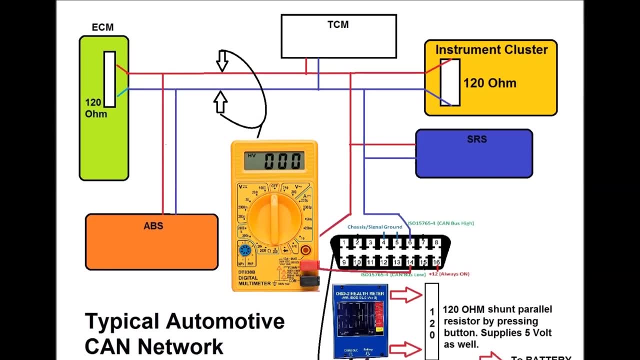 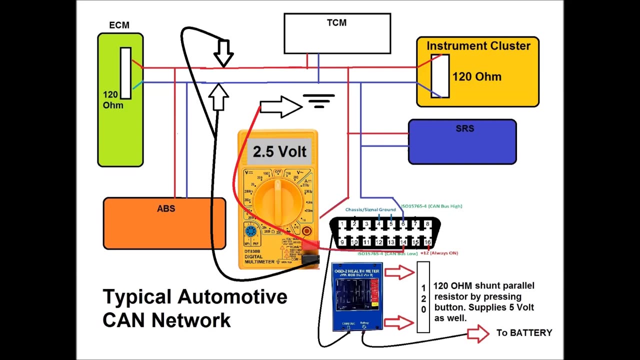 ground. so if you measure, measure across the uh CAN high and CAN low pins, number six and fourteen, it's going to be zero volts now, uh. if, on the other hand, you measure- and as you see now we change the diagram, uh, between ground, the actual uh chassis ground, which is, it would be pins of a pin number. 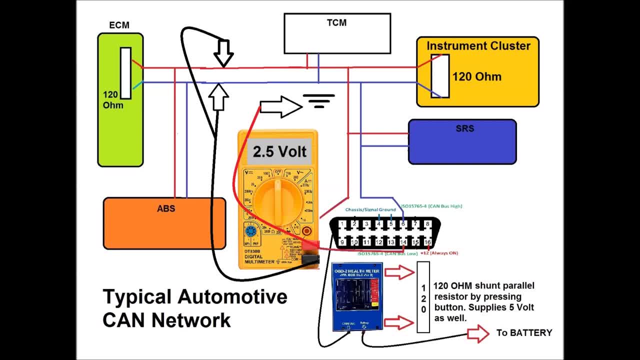 chassis ground would be pin number four. uh, if you measure between chassis ground and one of the uh, one of the wires- uh, either they can low or THEY CAN high- you're gonna see 2.5 volts. okay, so now going back to the uh, and this is basically what uh, the CAN uh protocol calls. 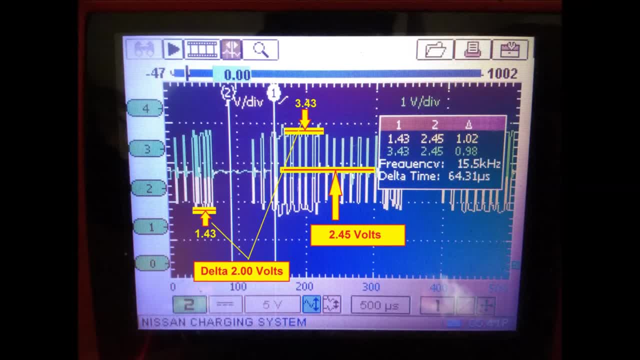 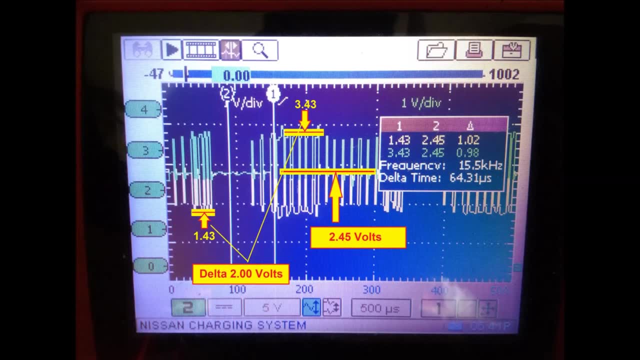 a call, for you have to have 2.5 volts between chassis, ground and uh, either CAN low or CAN high. now, because both wires are the same voltage potential between the can high and the can low voltage potential between the two línea will actually lower the request by one, not one. therefore, as you can see, in case if you see here as that, actually saying change the voltage, the one hassried, which returns to can low exposure, then you have to raise or detm Stewart, in order to add charge for the connected wires. you can the operate on a level and change the voltage for both, which is you cansa cũngñas acu. doesn't matter what has been calculated. you know you're seeing that voltage frequency and then, by the way, in all that when I flow, it has worked out. 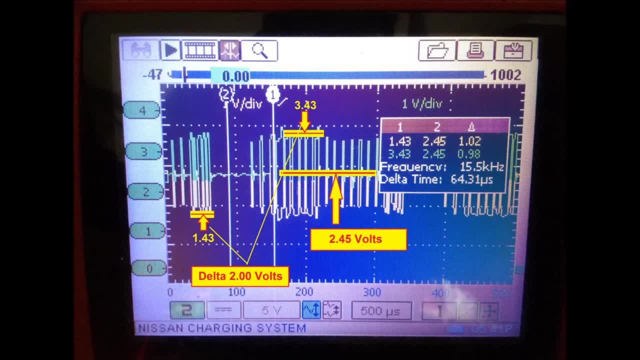 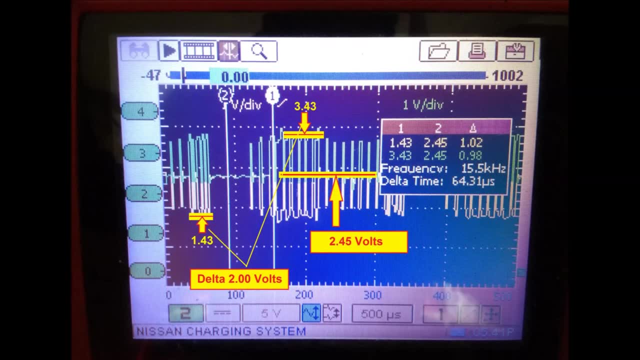 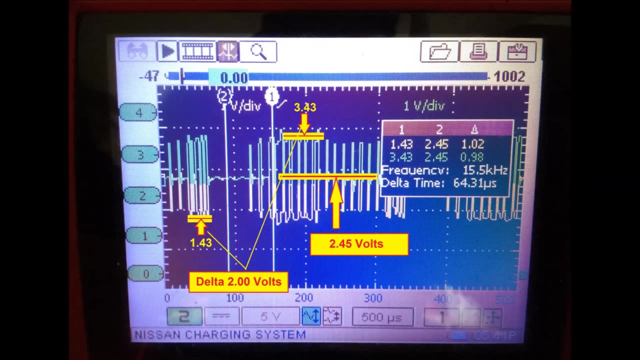 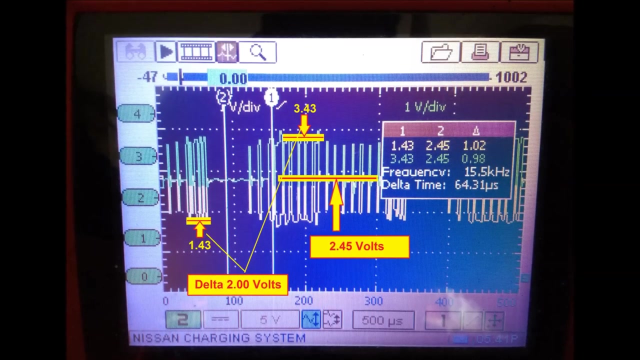 them. you see zero. okay, now we're gonna see on screen right now. this is, this is the. going back to the can. both both signal. basically this signal- the yellow one is the candle and the and the green one, the green half of it is that can hide. this is actually channels one and two of the scope, which you actually you. 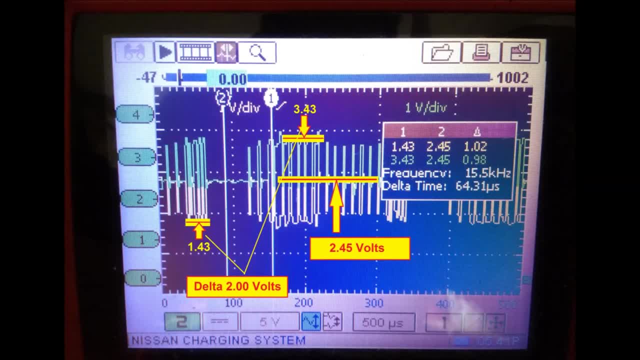 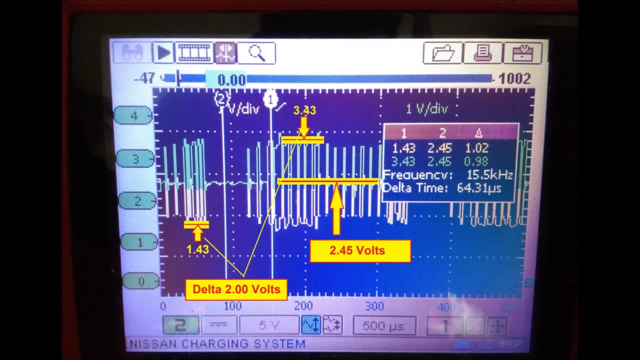 know if you're going to with a, with a unit that we have the OBD to health meter, you're gonna see exactly the same. oh so, basically, you're gonna see the candle and the can high. it's not really superimposed because they don't switch. 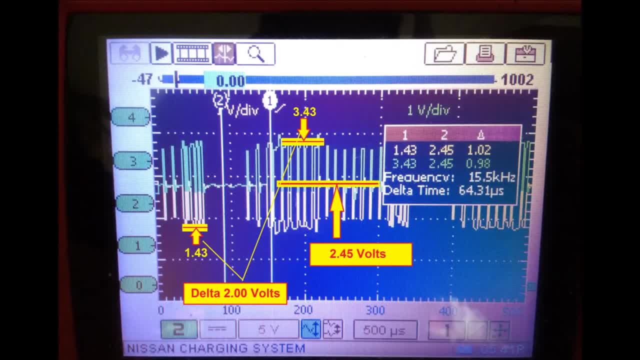 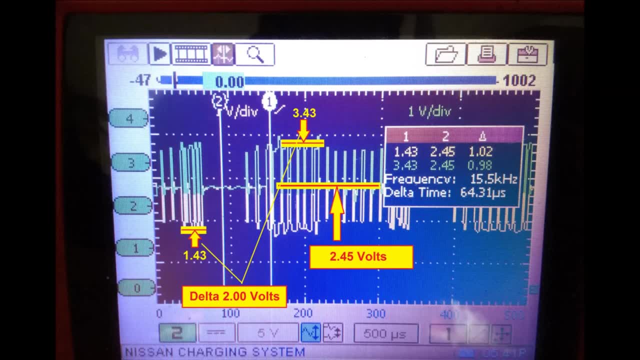 at the same level. they can't know. it's gonna go between 2.5 and 1.5. we're gonna see later on when explained that and the can high is gonna switch between 2.5 and and 3.5, between 2.5 and 3.5. 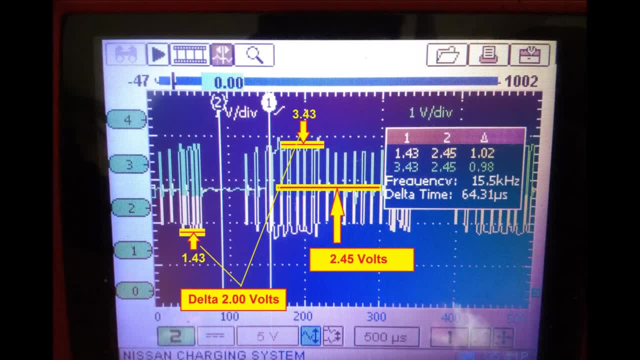 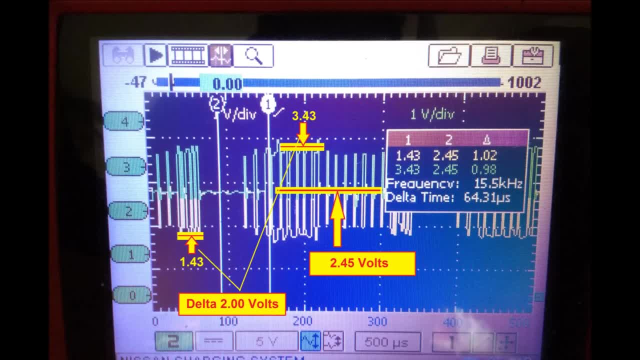 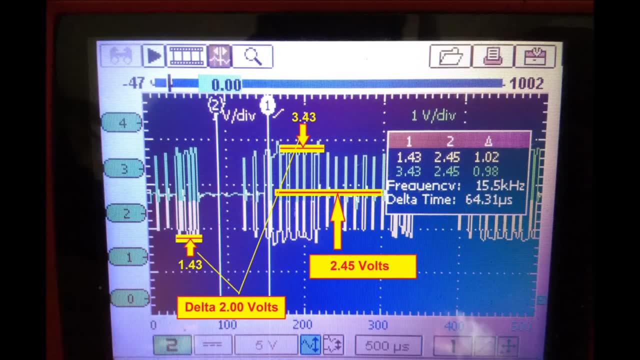 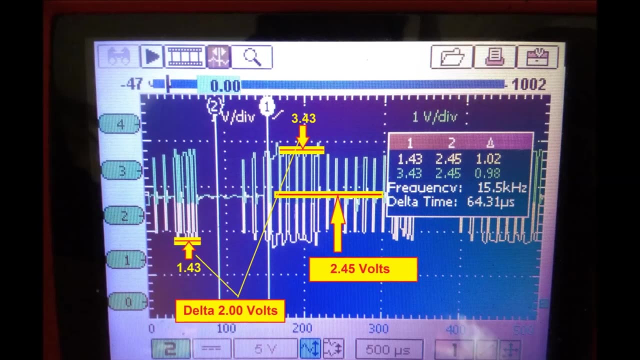 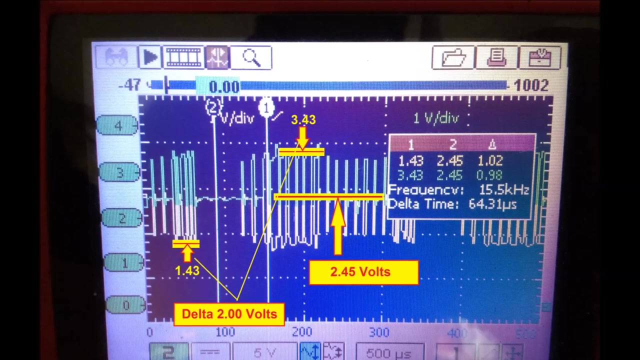 right now the can high and this is basically the what the signal says. the can high it's at 3.43 on the high side, 2.5 on the, basically on the on the resting side, and one point that the low can low is 1.43 uh on the low side and again 2.5 on the resting side. this is called uh the dominant. 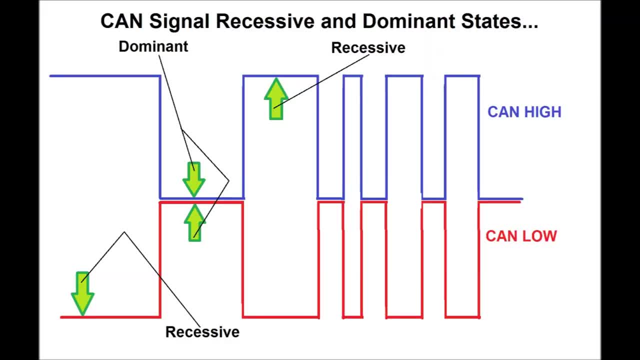 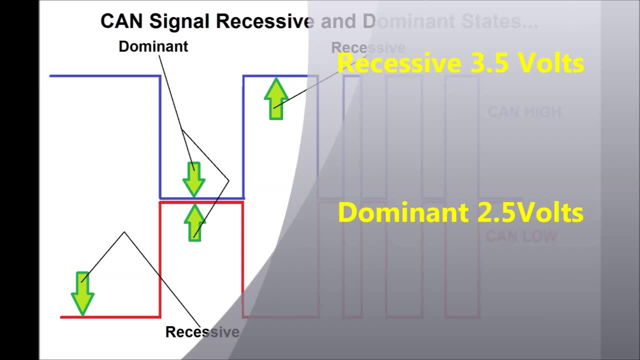 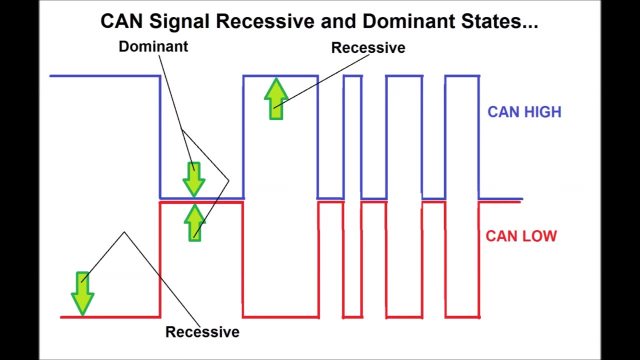 and recessive. okay, recessive will be the 2.5 for both signals, which is always at 2.5. in this particular case, it's actually 2.43, but this is doesn't have to be exact, but very close. okay, this is called recessive because it's always resting if the can is not communicating. uh, 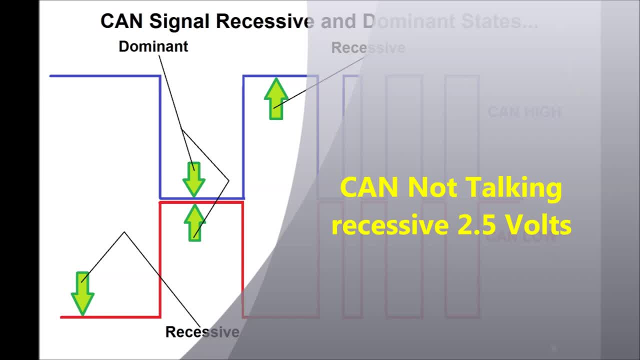 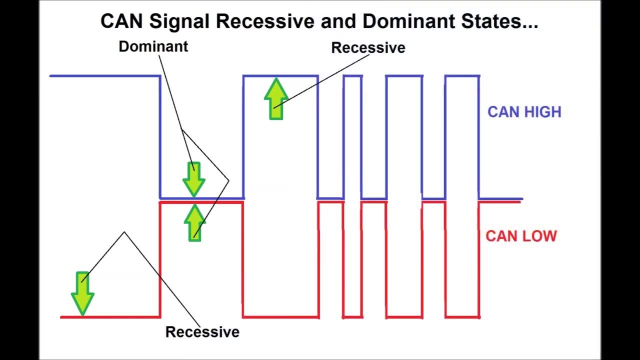 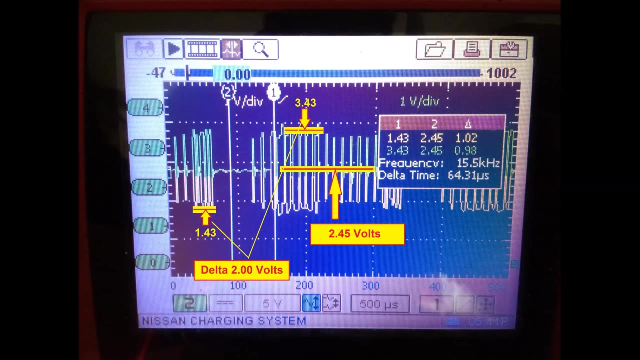 but basically you're going to have 2.5 volts. okay, this is uh recessive. the the dominant is when it actually switches either low or high. in this particular case, the can low is going to go to 1.43 in this, in this case, you know, or 2.43, i'm sorry, 3.43 on the, on the can high, which is the green. 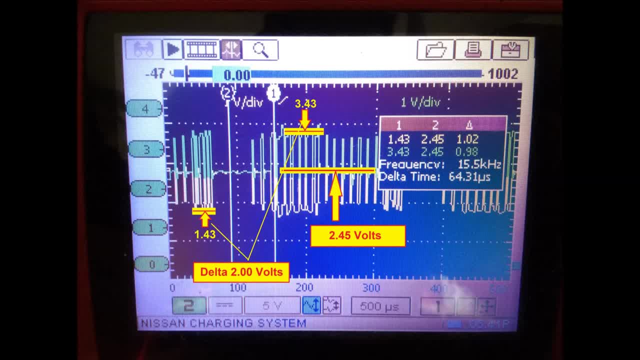 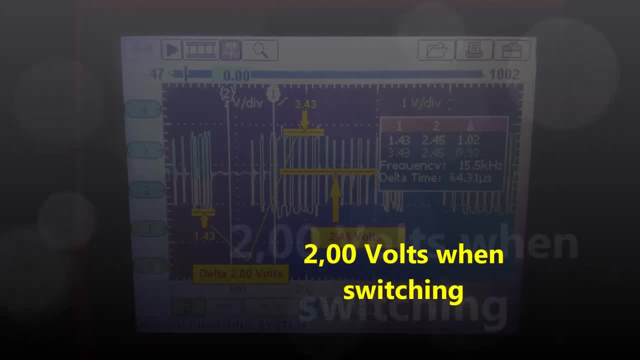 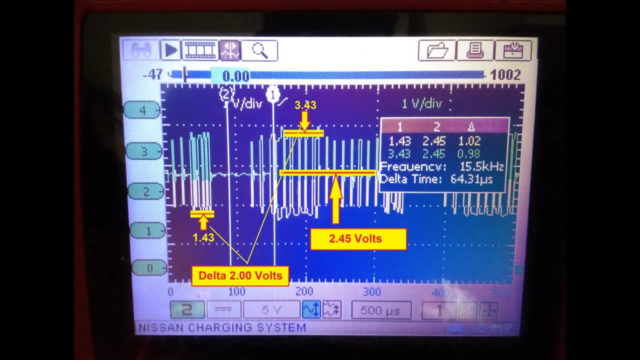 side, between the, the difference between both can low and can high when it's switching has to be two volts, otherwise the obd two, two, the, the can protocol, it's not going to work. okay, and this is uh, this last um uh diagram, actually the, the snapshot that we have here, it actually shows you that it, it says you know. 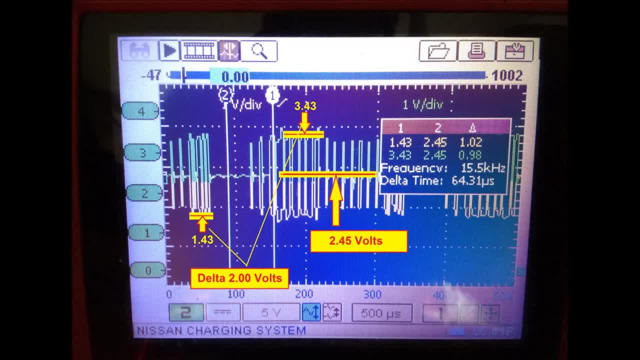 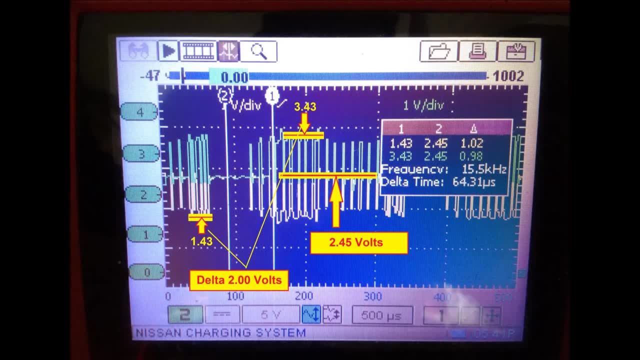 between the high side and the low side on both signals taken together. this is called the delta, which is a. delta means difference. the greek letter, which actually means the difference between the two signals, has to be two volts. you really don't care much about taking the 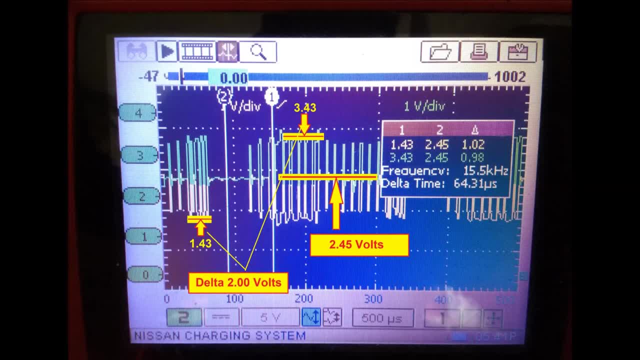 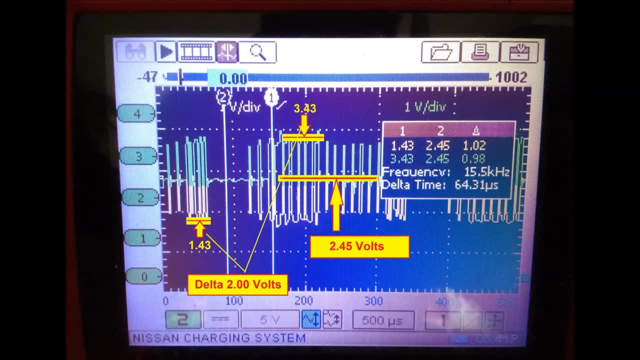 difference between the the two sides. um, because it's actually, you're actually going to see it, you know, like you see it right now, when you put a scope in in there, either our unit or or an actual oscilloscope, uh, so basically, uh, you know, and you have to be careful too, because sometimes, depending, 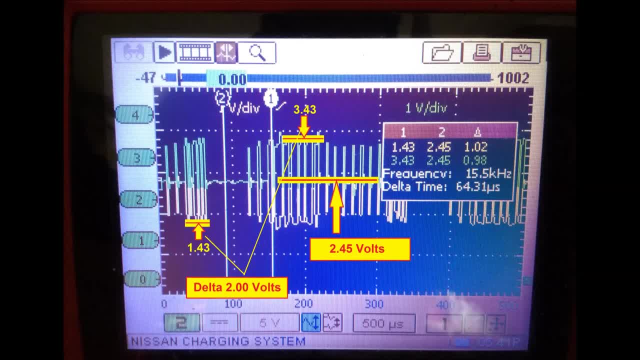 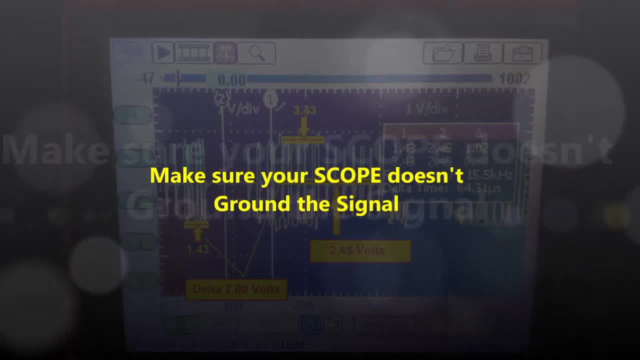 on the scope that you're using. sometimes the uh, the actual scope ground- is going to ground the signal. so be careful on how you do it, otherwise you're going to go nuts. you know, if you really don't know what you're doing, it's not, you're not going to damage anything, uh, but you're not going to. 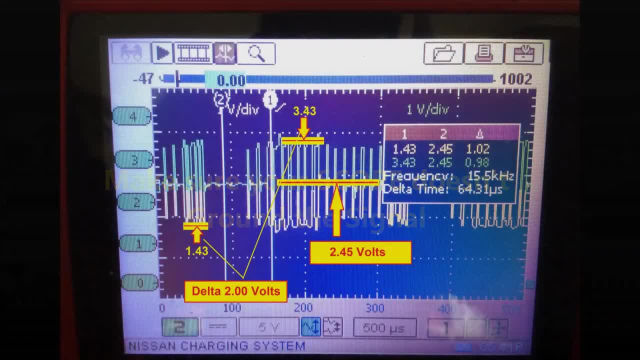 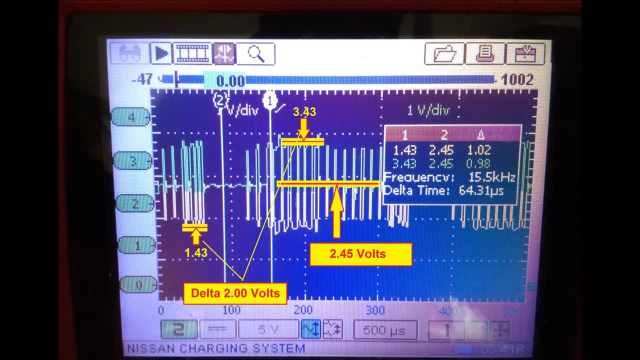 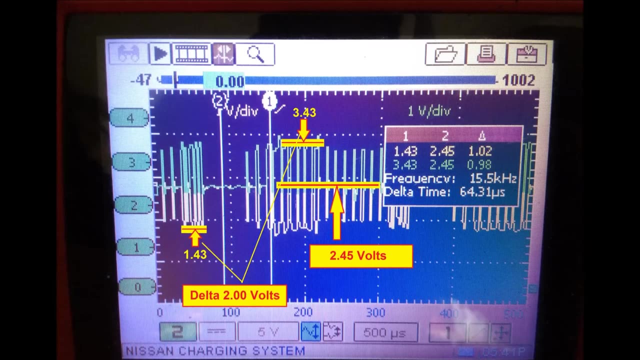 see anything on the on screen and then you're going to go crazy anyhow. so again, remember that the voltage between uh, the, the center voltage, uh, which is that's called the recessive uh can signal, it's always going to be 2.5 volts when taken between the chassis ground and the actual signal. 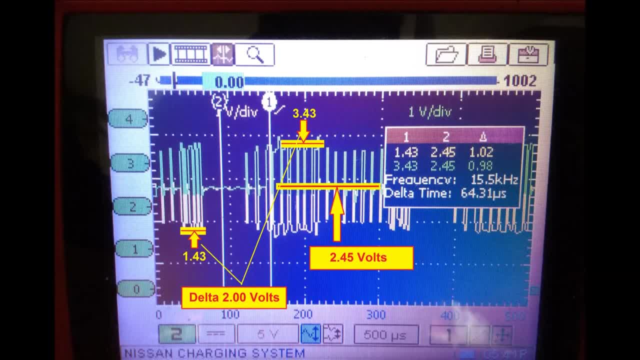 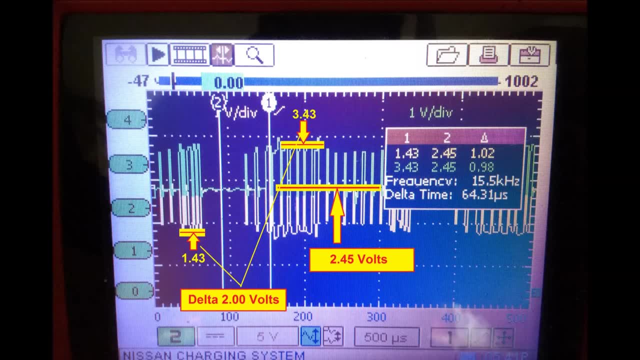 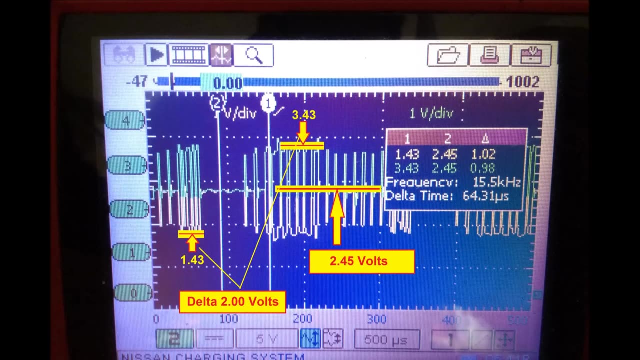 itself, uh, or which is the recessive, it's going to be 2.5 and the dominant, it's either going to be on the low side, it's going to be 1.43, in this particular case, 1.4. so, basically, in this particular example, we are 2.4. on the on the. 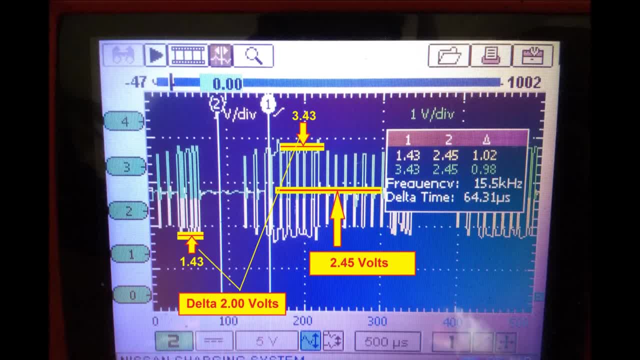 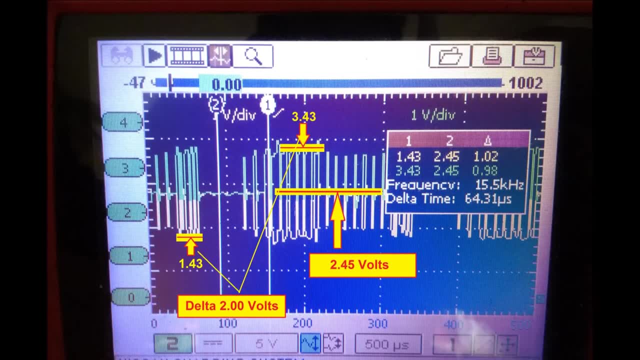 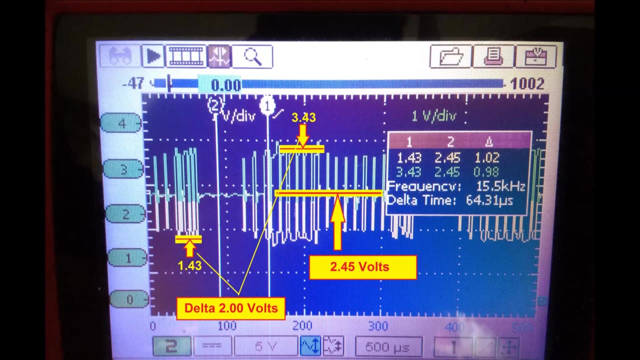 on the recessive supposed to be theoretically 2.5. so basically, theoretically 2.5 on the recessive, which is the center as you see it here, and the uh on the dominant, on the low side, on the can low is going to be 1.5. the can high is going to be 3.5. 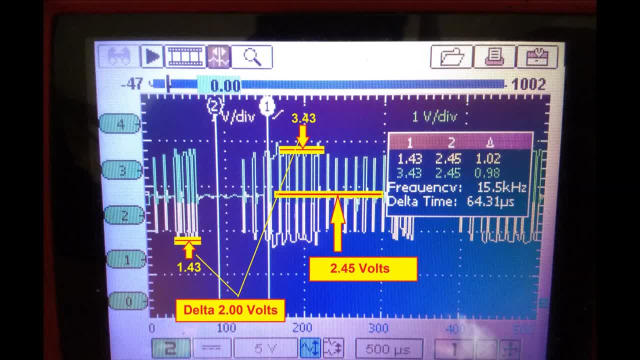 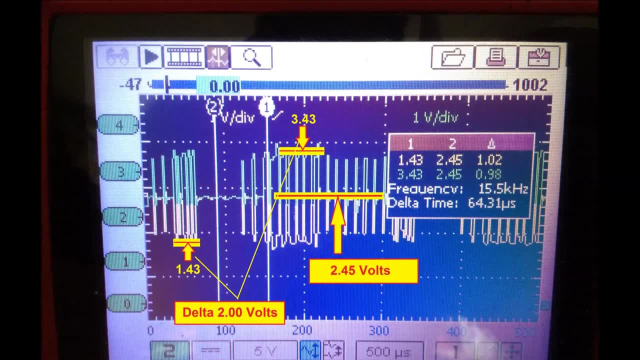 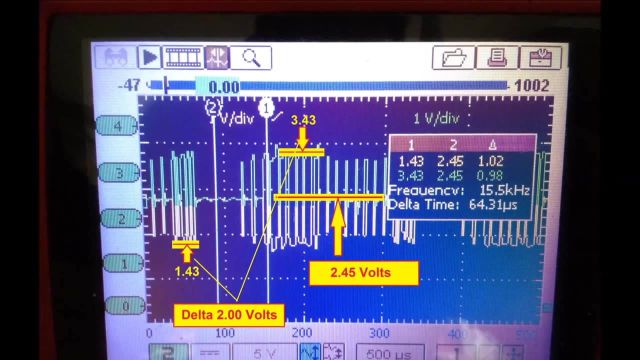 okay, this is really the theoretical behind the can protocol. uh, so between the two you have to have, as you see here, two, two volts difference between the candle and the can high, otherwise the can uh uh chips, you know the uh, the microprocessor inside that actually detect. 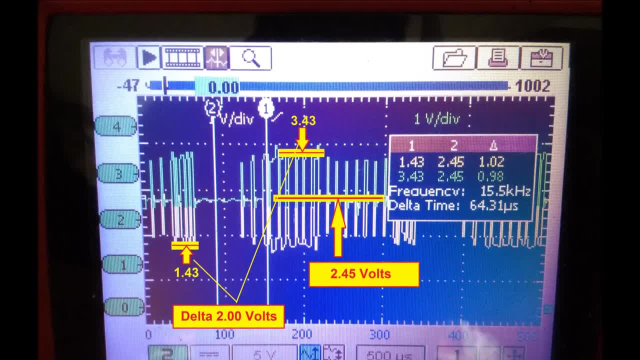 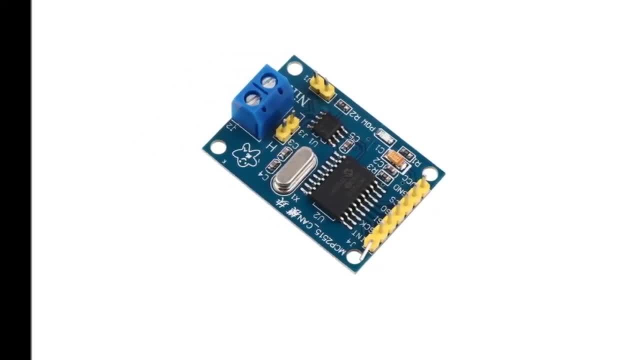 the signal is. they're not going to be, they're not going to detect the signal, and this is how you have to look at it. otherwise, and you could have, for example, a recessive of 2.5 or 2.4 or more or less, but then it's not switching all the way. the on the low side, the can low, is not going. 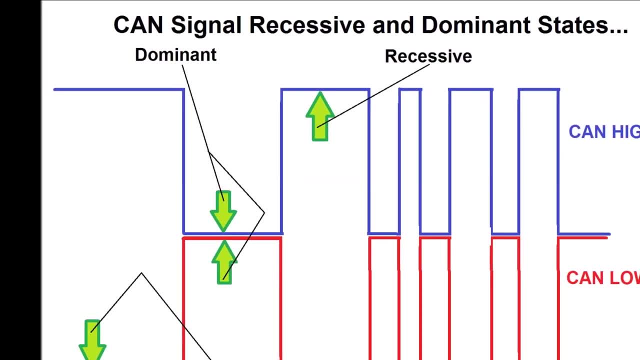 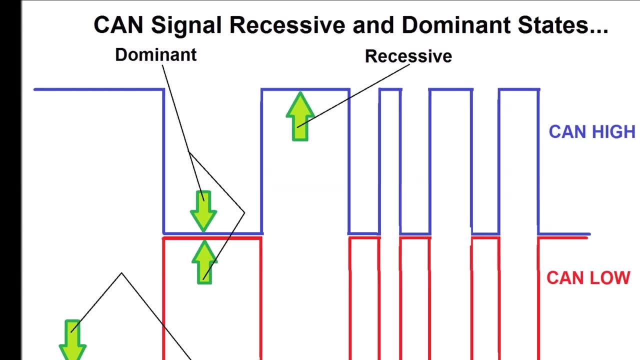 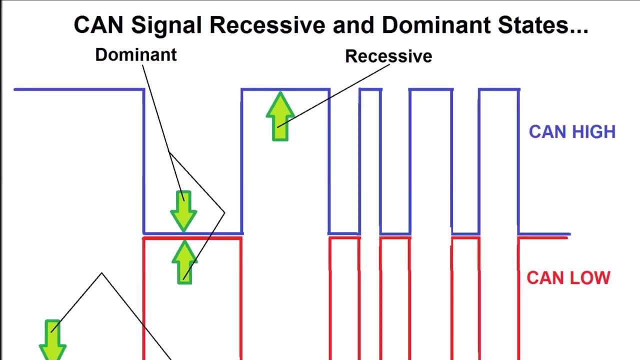 to it's not switching, maybe it'll give you, um, uh, two volts. okay, when it switches low and the can high is going to give you three volts. not three point, not 3.5, as you see here. then you know you have an issue. you could have resistance in the wires, uh, which is usually the case in one of the 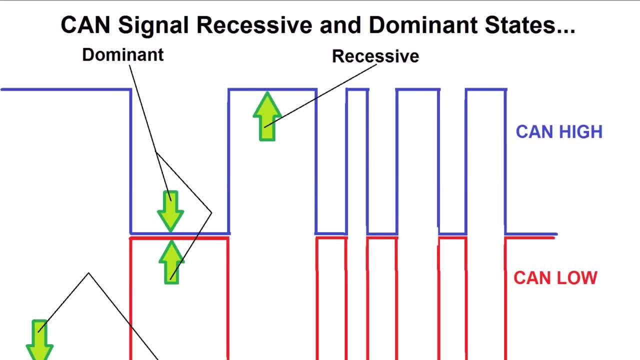 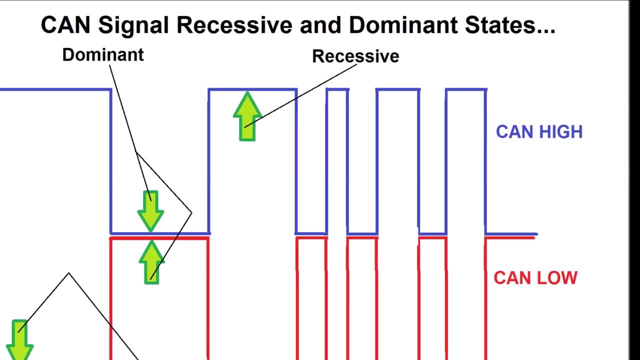 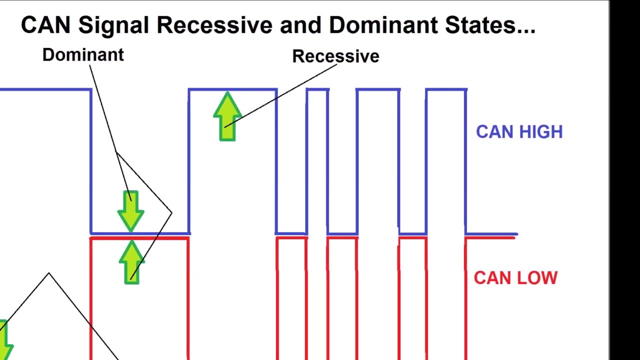 the nodes, one of the modules, uh, for whatever reason you know, maybe there's a lot of humidity where the vehicle is being driven, and this, this and that and who knows? okay, but definitely you can't have that. you have to have between the two signals two volts difference, otherwise the signal is not going to. 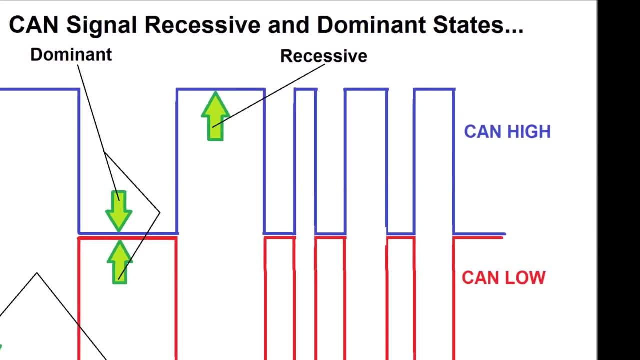 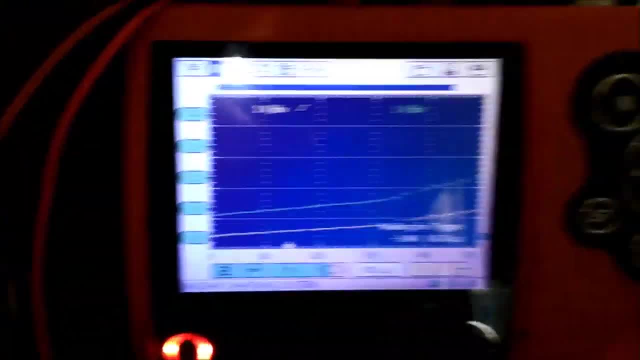 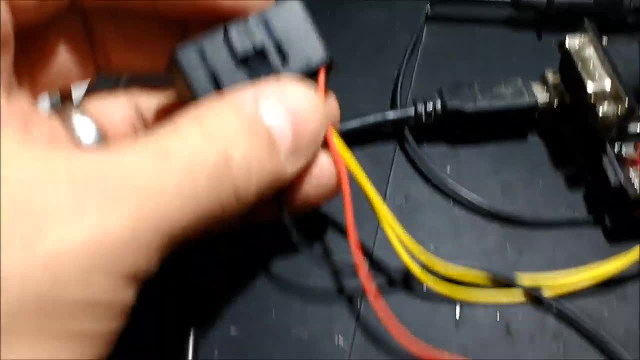 get recognized pretty much. now, as you can see on screen, we actually have a virtual network that we created, uh, with these gadgets that we have, they actually these are actually can uh transceivers that we have here, um which we actually we do a lot of experiments. 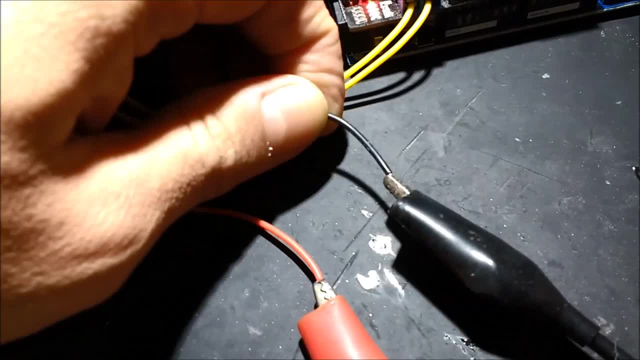 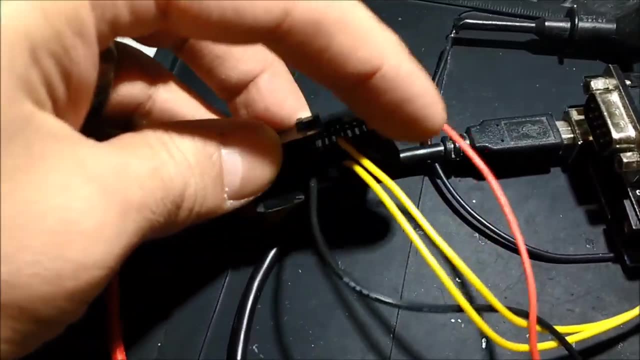 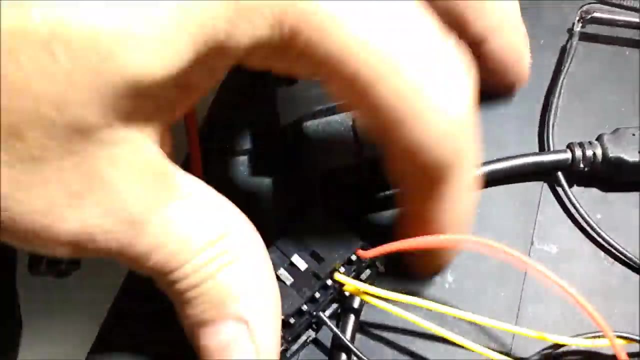 with these guys. now what we did is we took an obd2 connector and we rigged power and ground to it to be able to power the- uh, the little scanner that we have that we're going to use for testing. and then we the yellow wires that you see, it's actually pins number 6 and 14 for the can network. 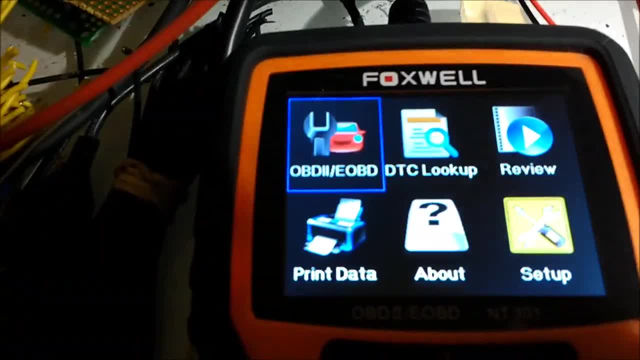 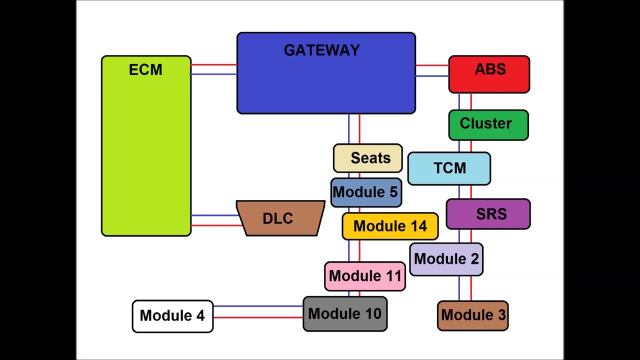 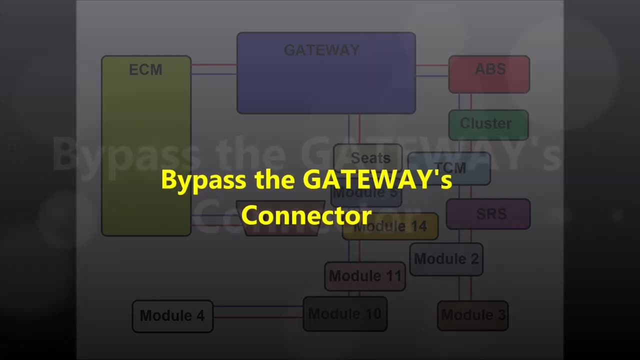 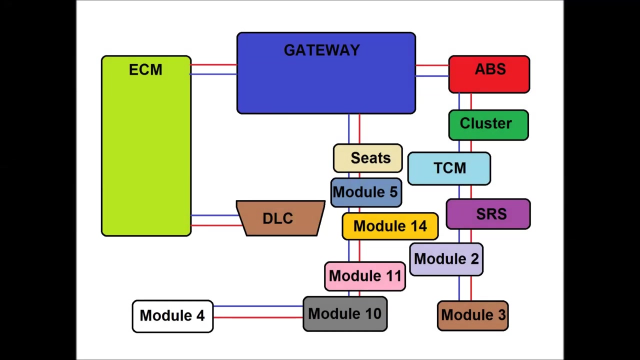 okay now, uh, some of you have the idea that if the vehicle has a uh- and we're really going to go into this very briefly right now- if the vehicle has a gateway, that, uh, all of a sudden, everything is lost and there's nothing you could do. that's not the case, okay, so, and um, as you can see, we're briefly, we're going. 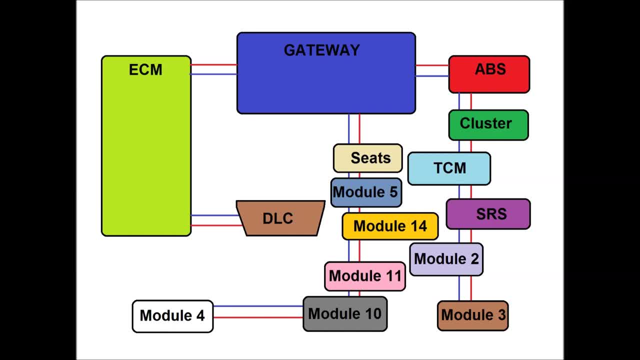 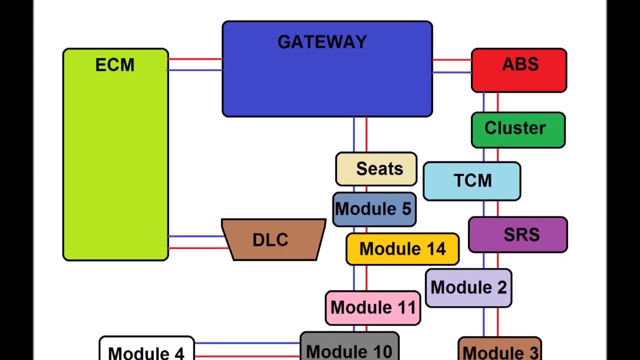 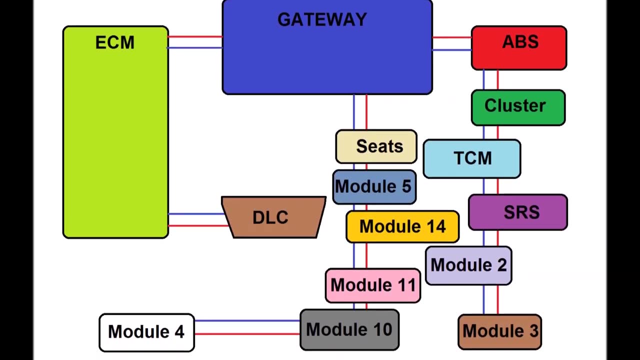 to explain this. we're going to do another video on gateways. so, anyhow, a gateway is uh, it's a, uh, it's a module that actually, uh, interconnects different modules together, uh, with the ecm and with the dlc connector. okay, so the gateway it's uh, basically, it's uh, something like a gatekeeper. that's why it's called. 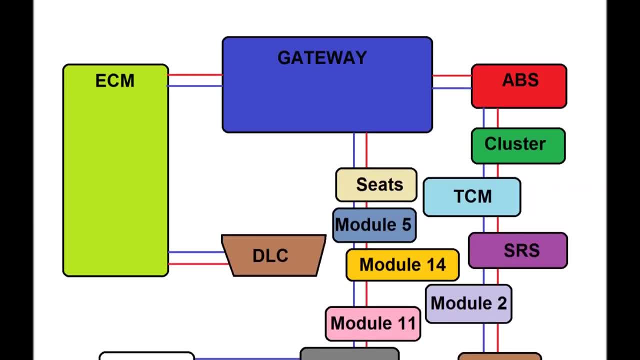 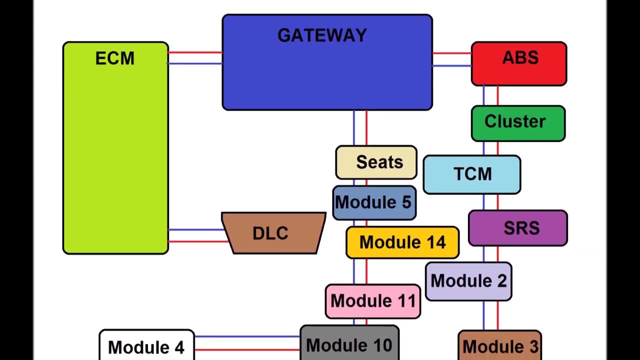 a gateway, and so all the modules are connected to the gateway and the gateway decides who has the access to the gateway. okay, uh, whoever has the access to the gateway has access to the other modules. that's not so in every single vehicle out there right now. they're starting to do that. 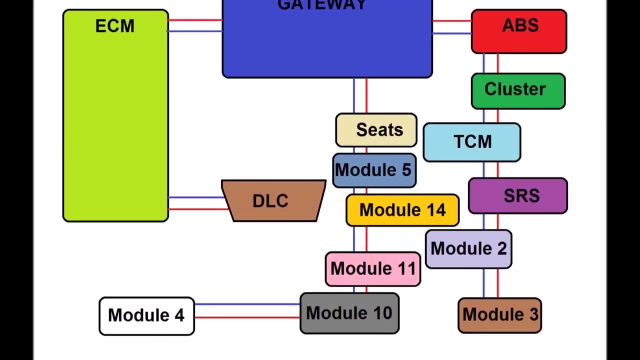 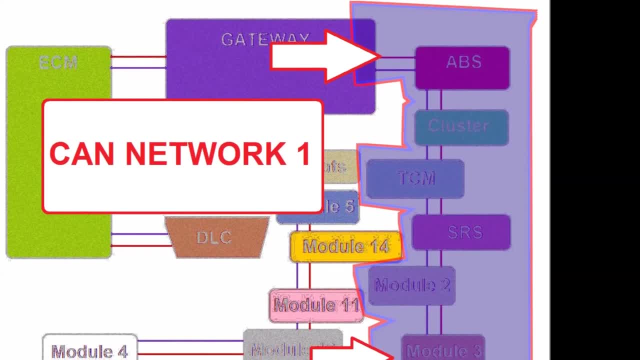 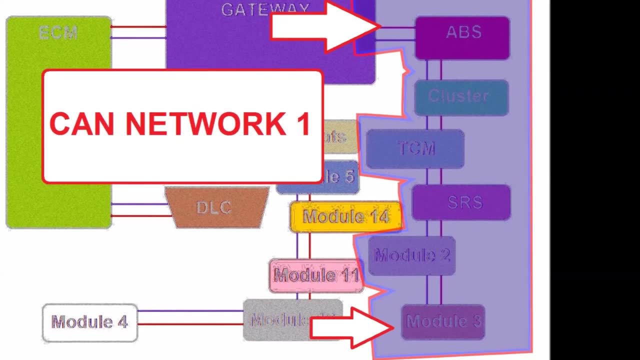 right now, as we speak, uh, this is the year 2019, uh, anyhow, so, uh, so, basically, a gateway is a gatekeeper for the different modules, and what it does, is it actually? uh, interconnects different speed modules. so you have the, the seat belt or the seat, not the seat. 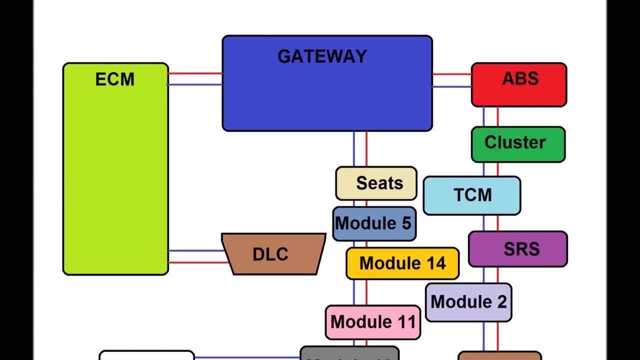 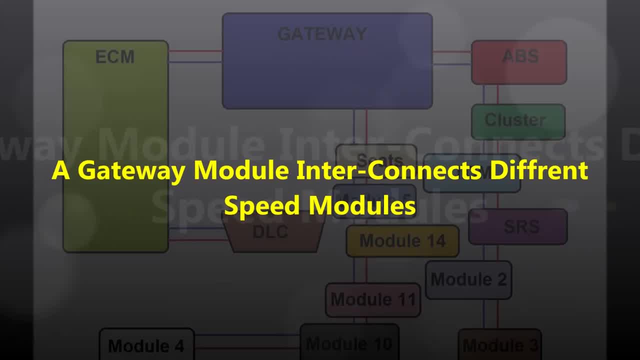 belt, the seat module, which is very slow- it doesn't have to be fast, so it's very inexpensive module. uh, that actually needs to need to connect with the ecm and everybody else. uh, you, you don't want to have it in the same uh signal that everybody thinks that this is because of security and this. 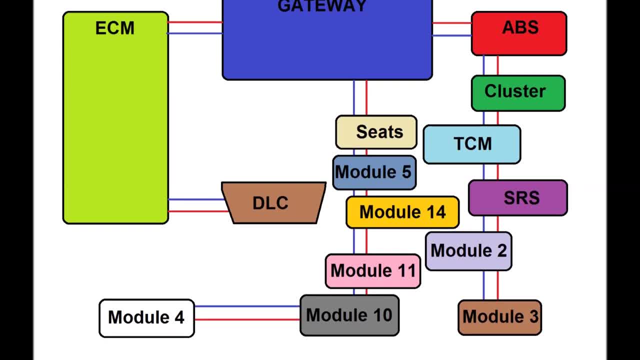 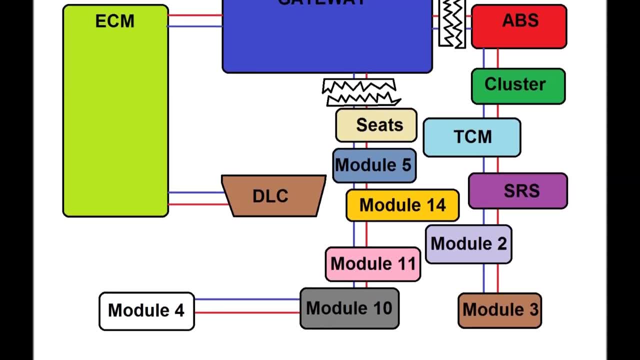 and that has nothing to do with security, because you're going to have to connect with the ecm and actually bypass the gateway very easily, as we're going to explain. so, basically what you do, if you want to have access to the can network, you're going to have to remove the gateway and connect. 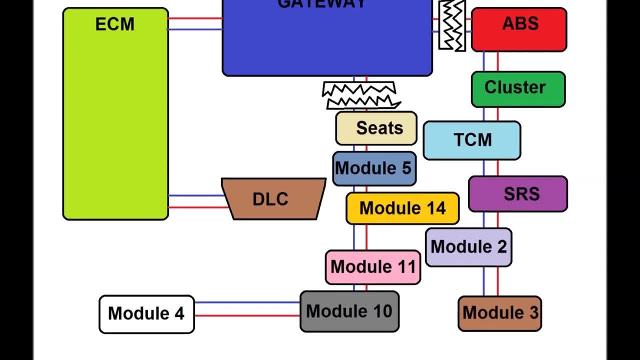 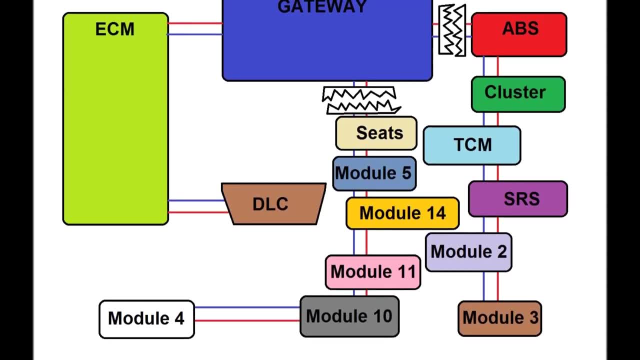 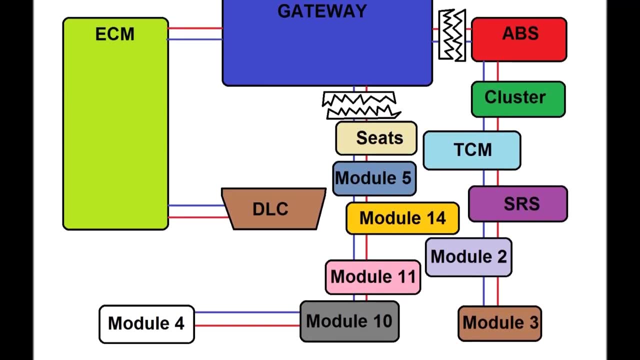 to the two uh, can uh wires: the, the candle and the can high um uh, on the other side of the gateway, as you can see on screen right now. so the gateway, you know, restricts access to the other module unless you have the right scanner. uh, but you don't, you know, like for example, on chrysler vehicles. you, 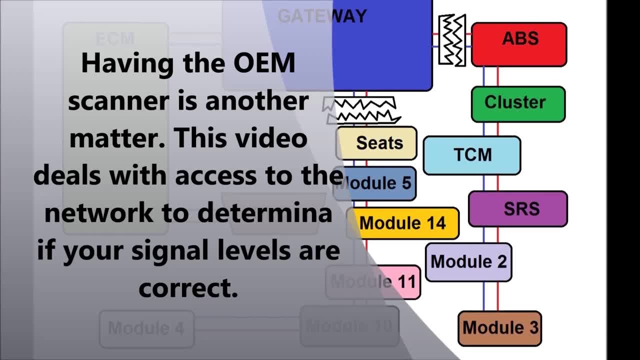 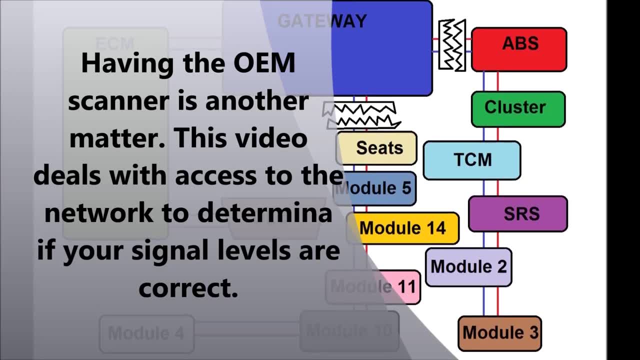 have the gateway which is right behind the radio, uh, and basically you have access to, to the, to the one wire. you know that the, the can uh signal wires, the can low and they can high, and once you have access to those, then you can actually access whatever module uh you want, that's, if you have. 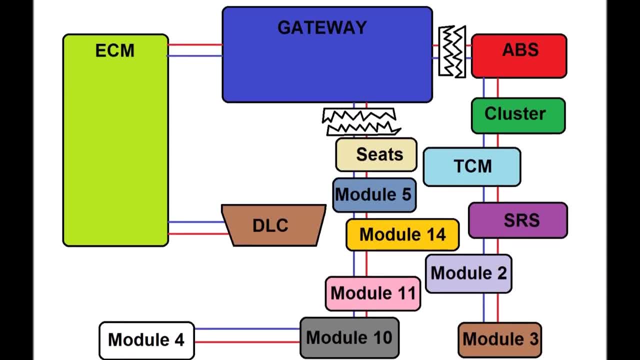 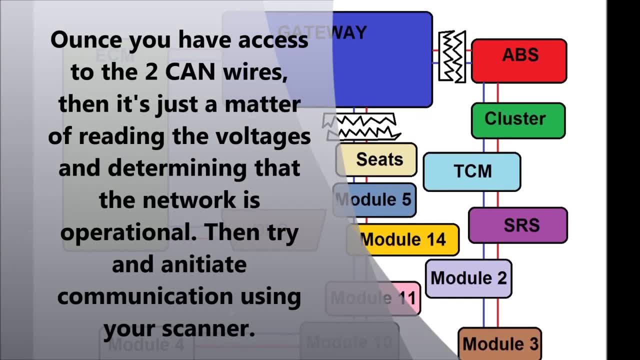 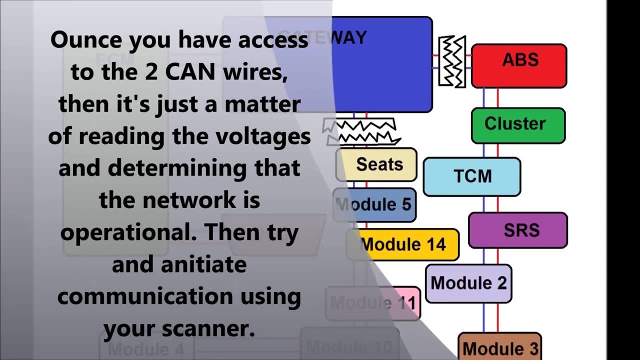 the scanner that actually communicates with the gate. but if you just want to see that you know that the network is running properly, uh, that you can actually. actually you could do that manually by going to into the, into the wires necessary on the vehicle that you're working on. but just trying to explain to you that the gate 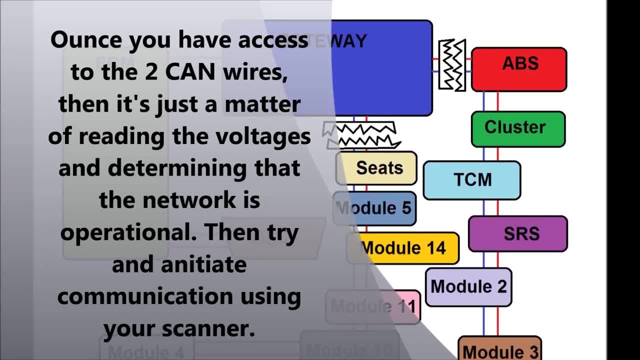 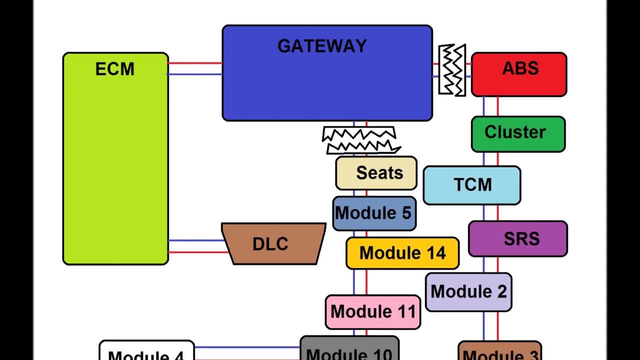 once you remove the gate, put the gateway out of out of the the picture, then you actually have access to the, to the can y, and you can actually do whatever you want. if you want to connect the scanner to it, fine. if you just want to see if you have the termination resistor, which is really what, 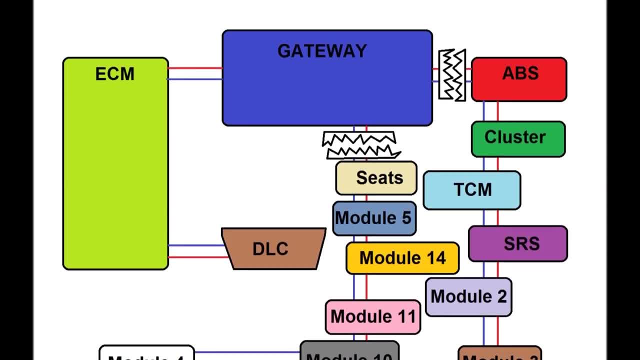 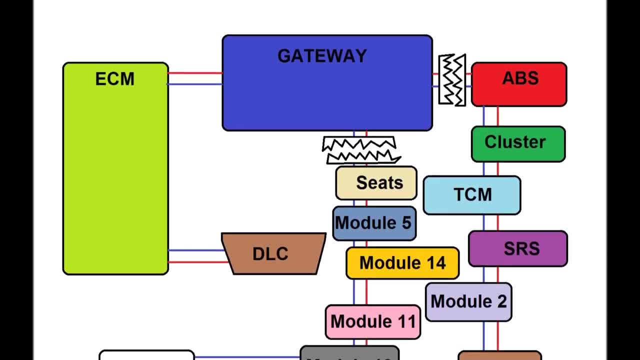 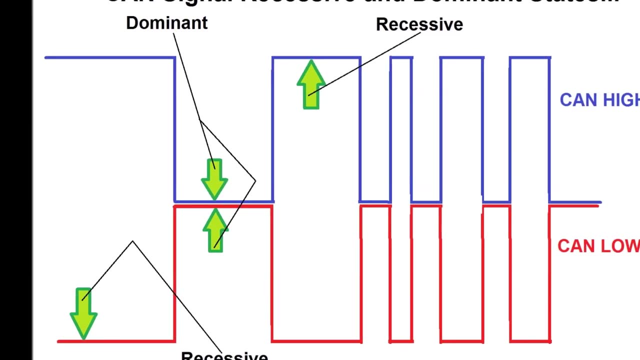 we're talking about here. uh, that's what what this video is really for. and then you can actually do that on the other side of the gateway if you know that you have the termination resistors, fine, and you can see that the signal is, the signal is okay. uh, then, basically, once you know that, then your 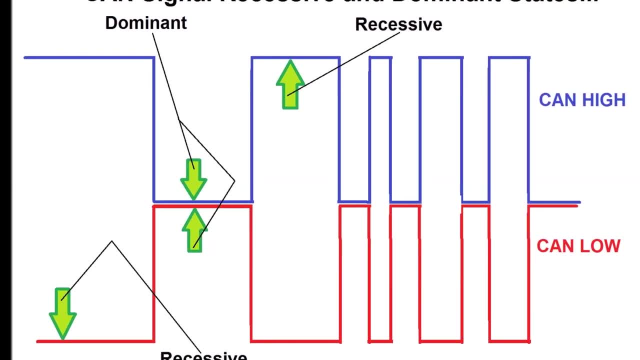 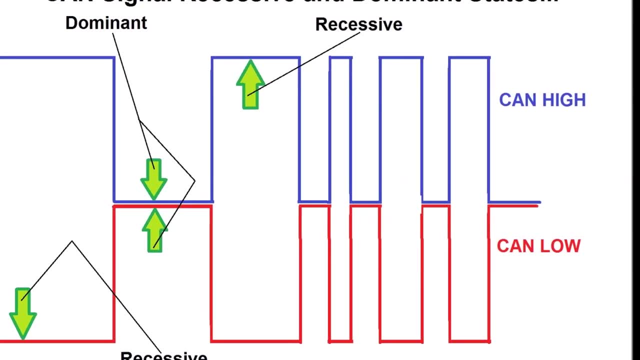 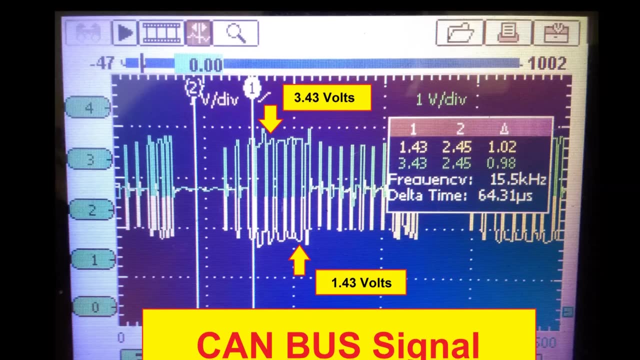 problem is: it's, uh, whatever problem with the specific module that you're trying to communicate with, uh, not necessarily a problem with the can network. uh, which is, again, this is the purpose of this video- is to make sure that the actual physical um, uh, the physicality of the of the 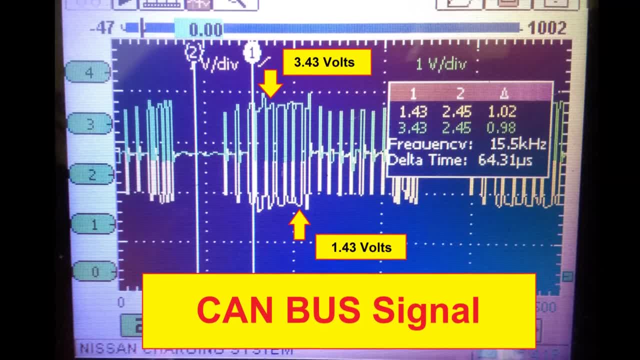 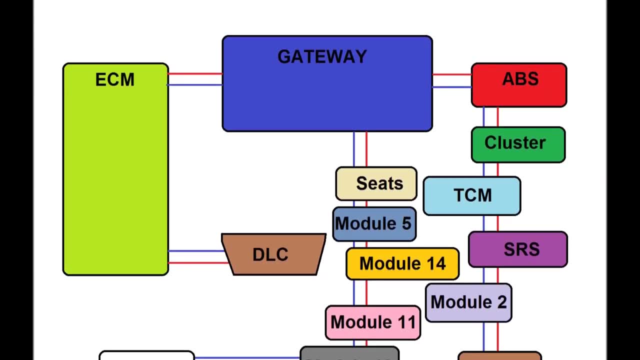 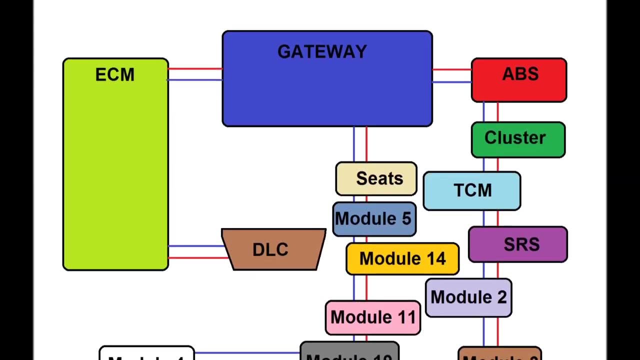 network. it is there and basically, you, you're looking for the termination resistance. it has to regardless, you know, and in this particular case, if you have a gateway, as you can see on screen, you have interconnections between these guys. they, we have actually three, three networks on screen right now. the one with the ABS is 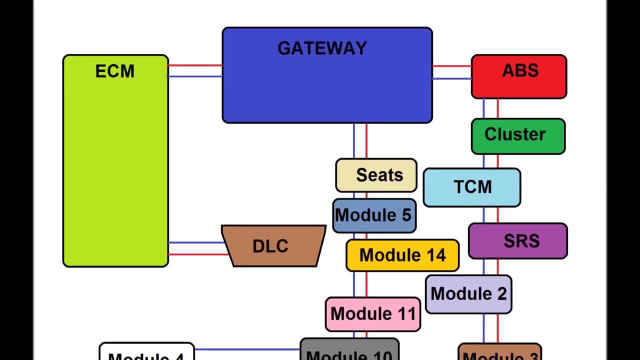 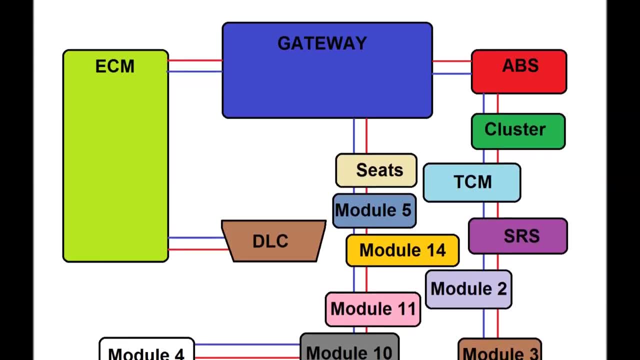 one network which has the ABS, the cluster, the TCM, and then the and the other modules. and then you have the other one which has a seat: module 5, 14, 11, module 10 and 4. that's another network. they're all interconnected to. 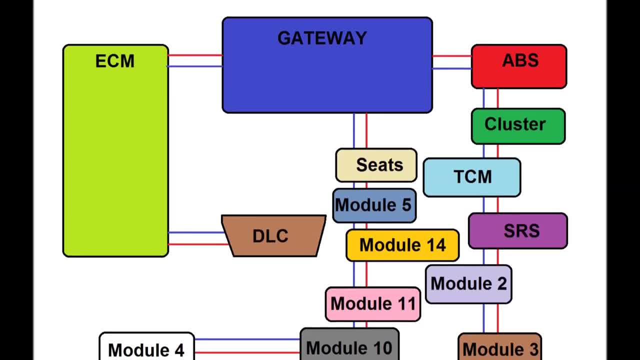 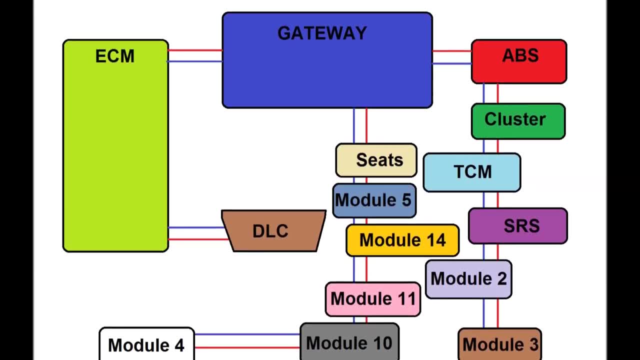 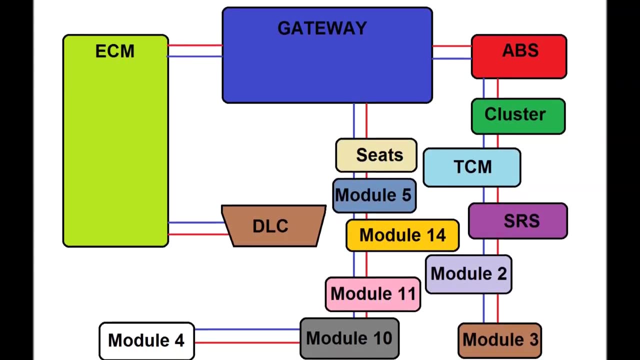 the gateway and each one has to have a termination resistor of 120 ohm and two of the- in this particular case, for example, the, the module, that network that has the ABS on it. you're gonna have a termination resistor on the gateway itself and you're gonna have it terminate- not necessarily, but usually it. 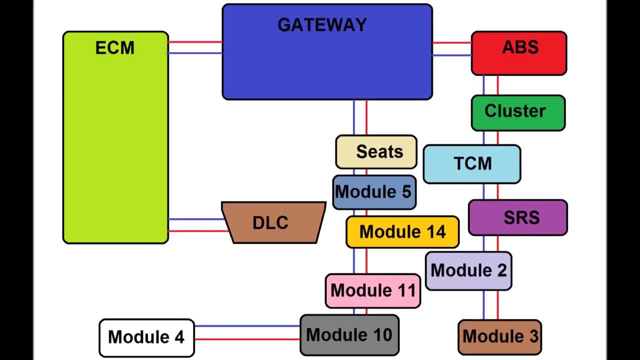 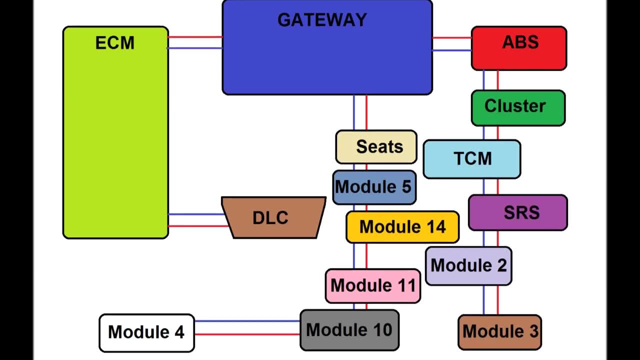 does, and another termination resistor, for example module 3, which is all the way at the end. it could be in any of the others modules and you have to find out which one it is if you don't have that termination resistor. if you measure between those two and that particular network, if you 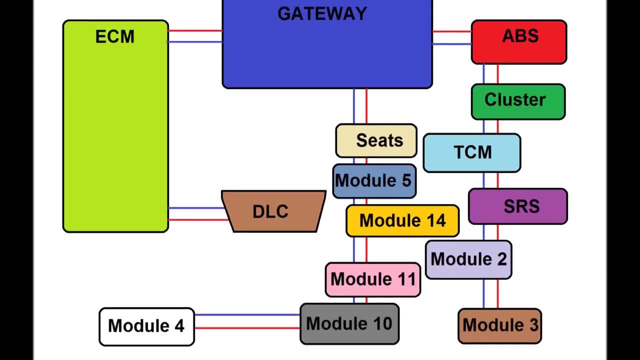 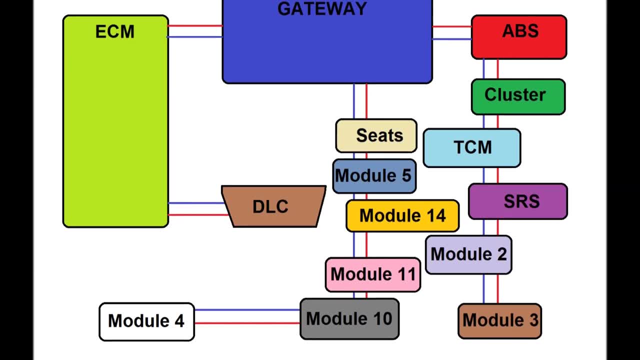 measure between the two wires. they can't low and they can't high. you don't see 60 ohms, remember it's 120, and we have to have two of these. okay, and that between the both of them. it's a, it's a, it's a 60, 60 ohm, but each one is 120 ohm resistor. 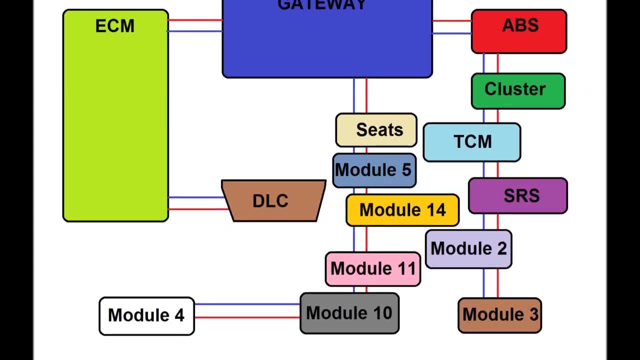 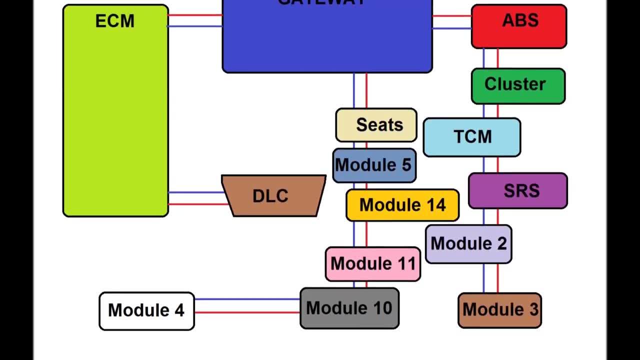 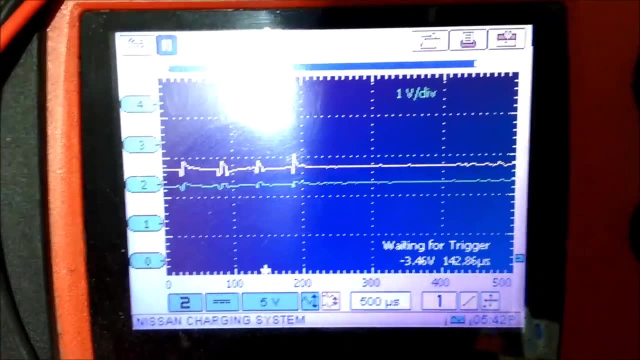 so where is it? that's up to you to find out, and some, most often, times is not easy. okay, and this is the issues with when the connection is off and the board you always have to fill in once the batter discharge is off and you don't. you don't see problems with the, with the. 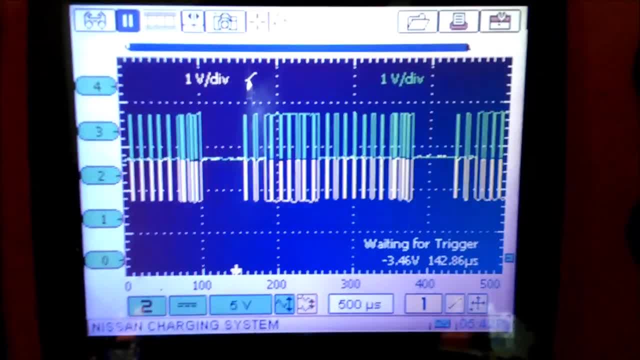 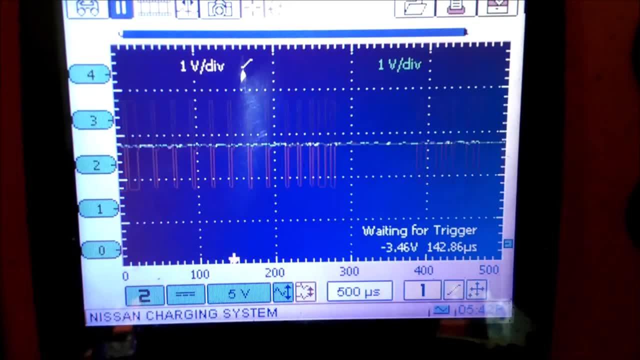 communication with a can, as you can see on screen. this is life. this is actually the scanner, trying to establish communication when not necessarily connected. the virtual network that we have will give you the voltage level, some will give you the termination resistors, but it's not. you're not gonna. 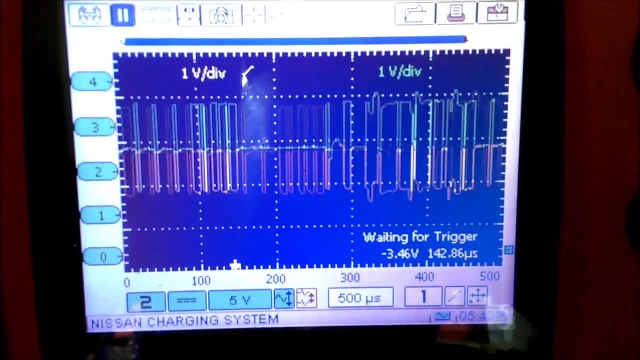 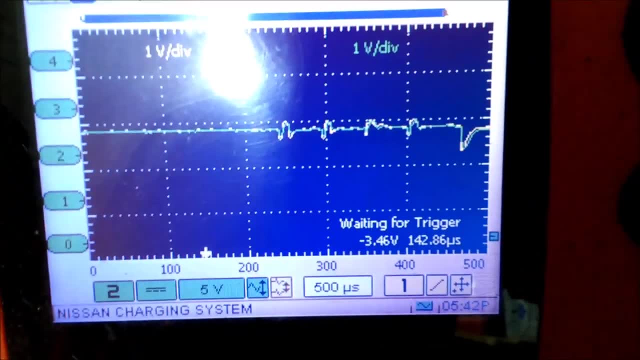 see anything because we're not dealing with the over, dealing with the can network, we're not really connected to a car and we Diagnostics on a regular vehicle. you're not, you're not going to look at, see, you know, watch these Pulses in there and say: well, that pulse is for the ABS. 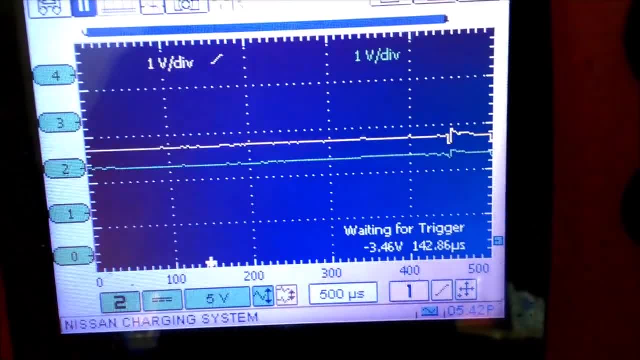 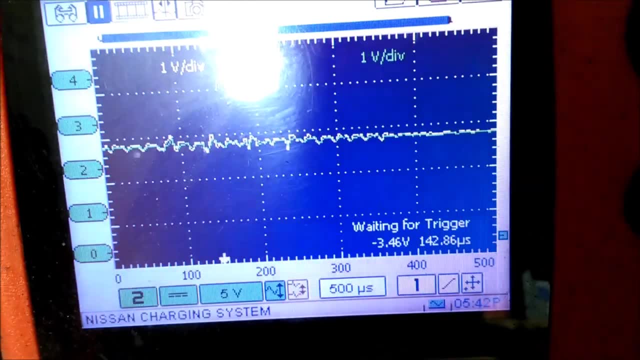 I recognize something. you never be able to recognize that pulse. you need a network analyzer for that And it's really you don't really need that. you don't really care What the pulses are, the for that you use a scanner and you try and establish communication. if you don't have, if you have a problem. 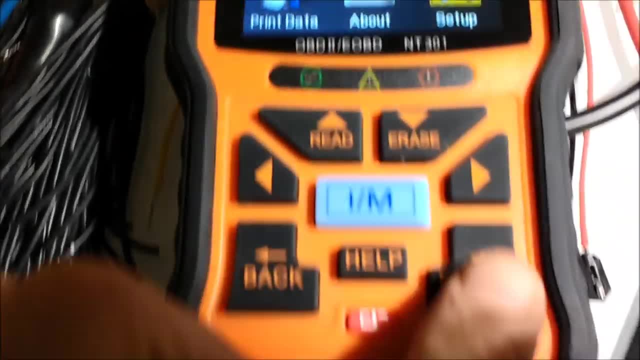 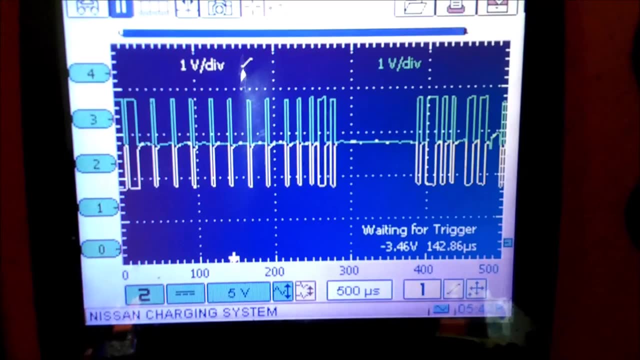 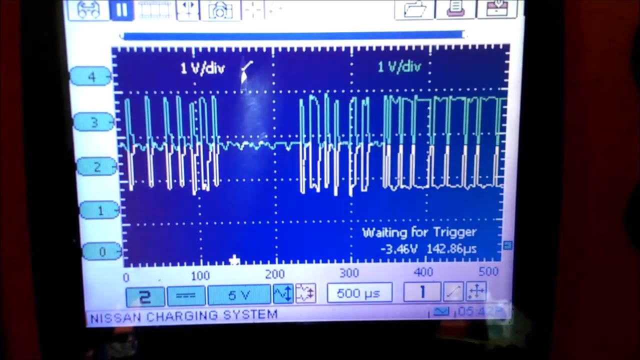 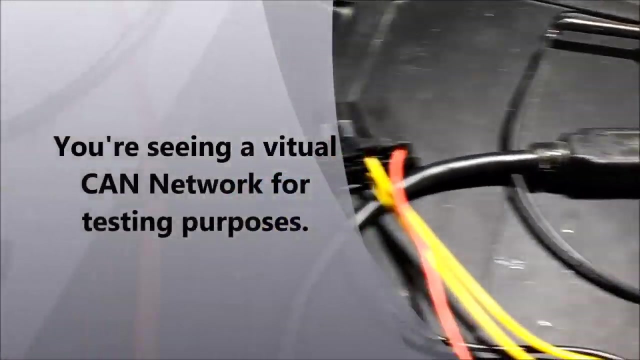 with the I don't know, for example, the ABS module. okay, and the ABS module, it could be at the seat belt module or the seat module, that, the power, you know, the power window module, whatever, and You basically you have no community. you try and establish communication With the with a module that that's, that's not communicating and usually what you have is you're gonna have faulty codes. 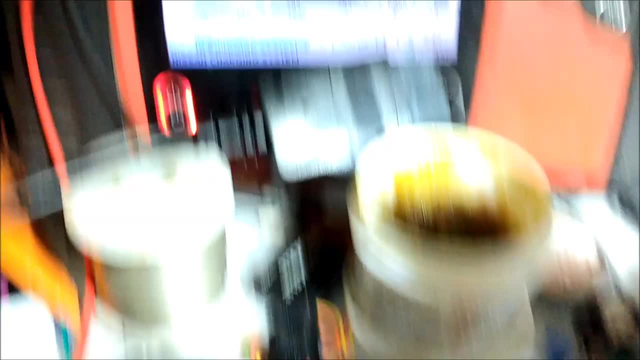 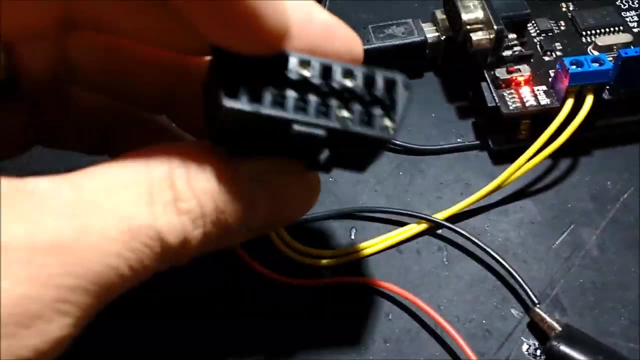 on the, on the other modules- No communication with the ABS module, for example, and everybody Else is going to have no communication with the ABS module. So if you look at the TCM, the transmission, if you look at the ECM, you look at the- everybody else- no communication with the ABS. 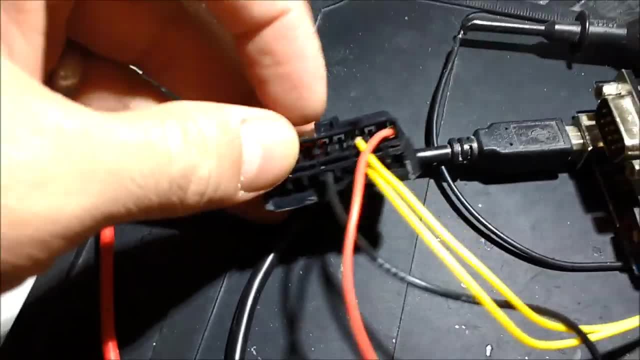 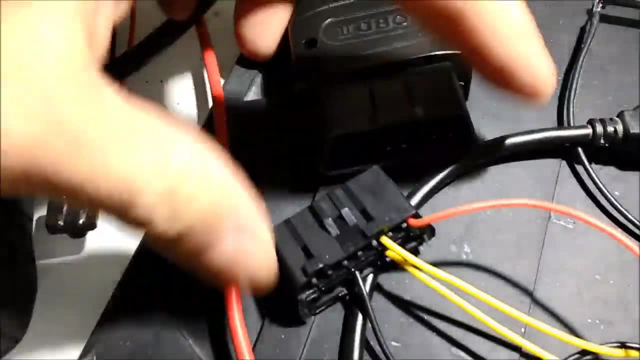 Module, so the ABS module is not communicating. so you look at the network where what it's a connected to And if you, if you definitely have determinations in there, the 60 ohm between the two, the can low and the can high, and you have the voltage. 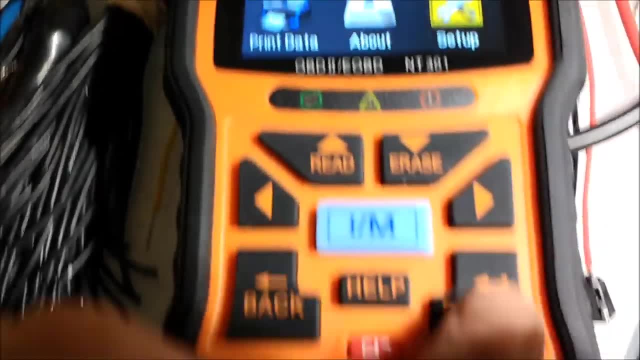 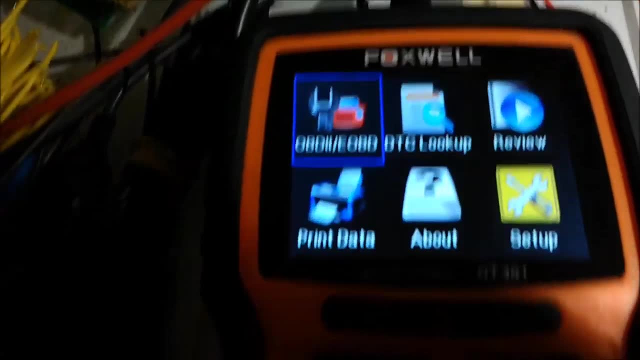 2.5 volts between ground and either either one of the Oh, they can. okay, the can low and the can high. then you have your physicality, is there? That, basically? what you have to do, then, is find out why you don't have communication with the ABS module. 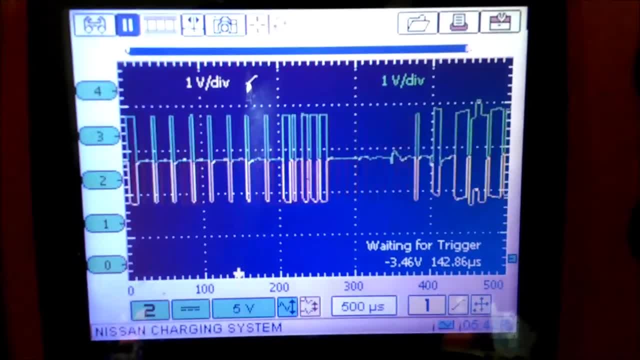 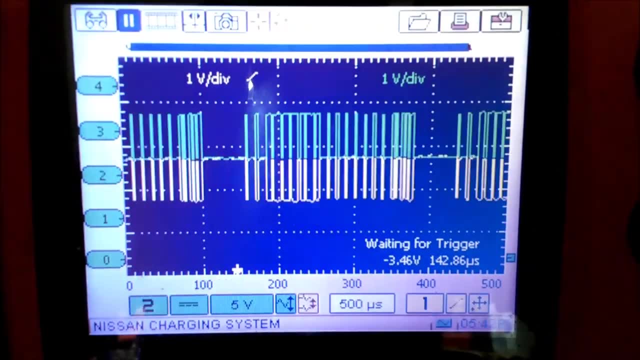 It could be the ABS module itself is shot, It could be the the wires, or one of the wires is cut. you know somehow broken and you have no communication or whatever you know, but you deal with it. then you know that your, your problem is not. 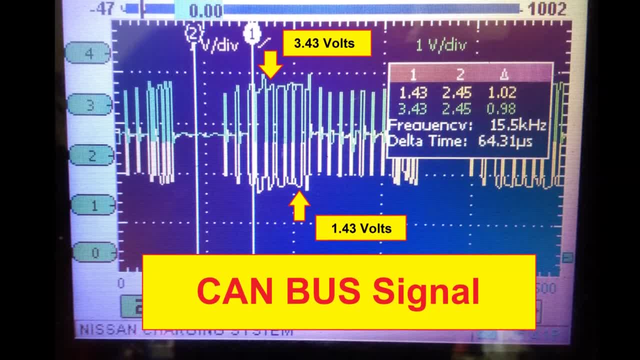 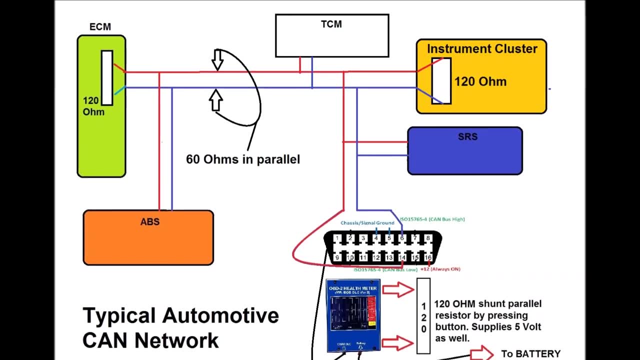 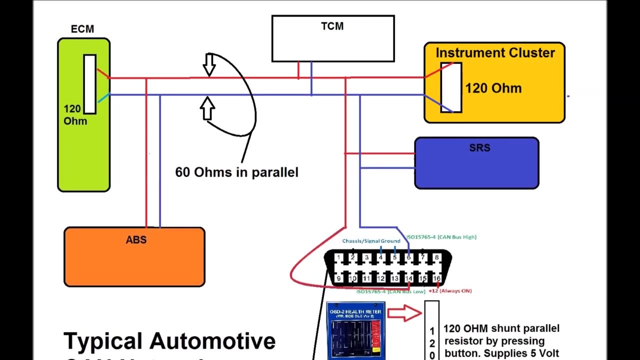 necessarily a broad problem with the with a can. if you have No, no, 60 ohms between the two cables, between the two wires, can low and can high, Then you have to start tracking why, and in which case you're not going to have communication with a bunch of the modules. 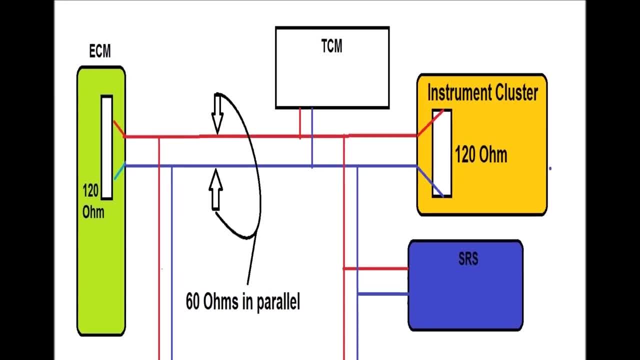 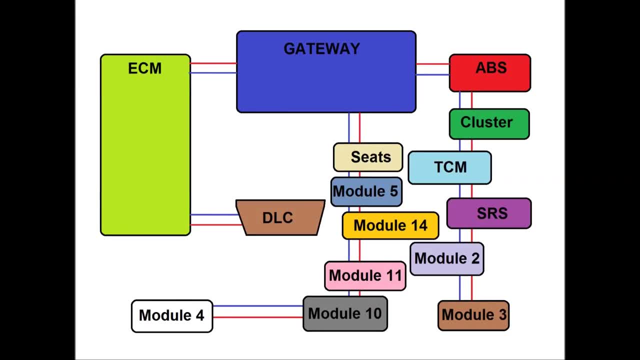 going back into the, the Gateway that you saw before You're gonna, then you have to find out, you know, how many networks do you have? because you could have three, you could have two Or three networks and if each network it's going to have a. 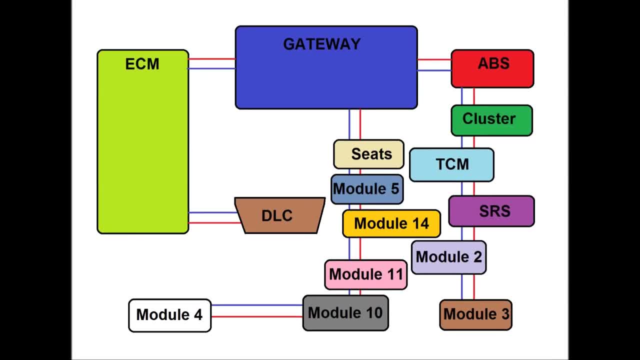 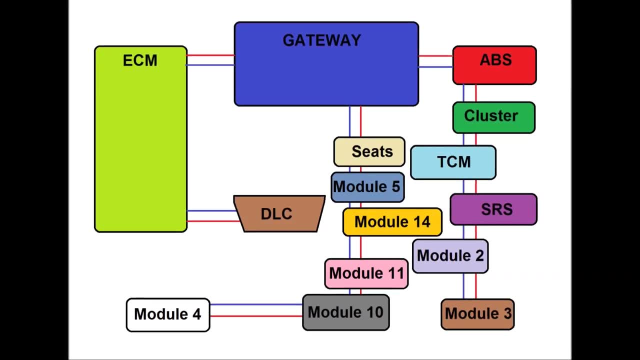 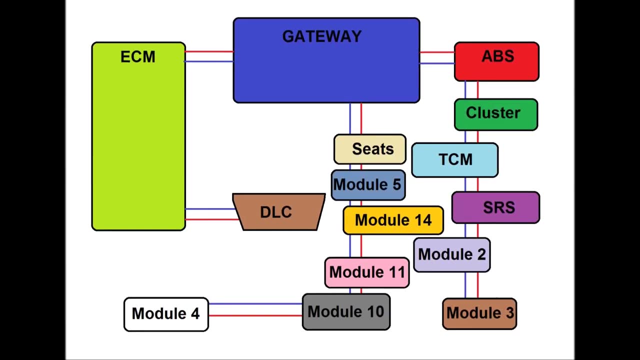 specific Bunch of different modules and you have to find the modules They try to establish communication with and find out why you don't have communication. usually if it's a broad problem, You're gonna have no communication with all the modules on that particular, And sometimes the gateway itself is shot and it actually has communication with the other modules but not with the network. that that's defective. 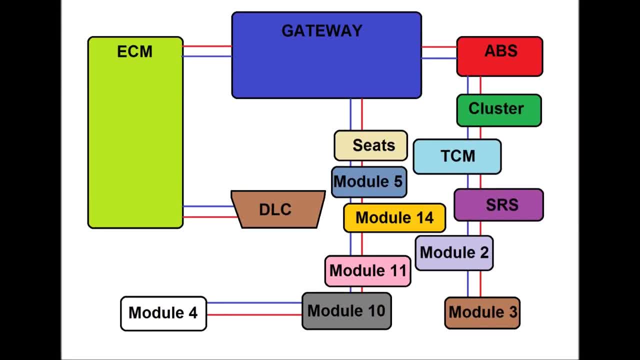 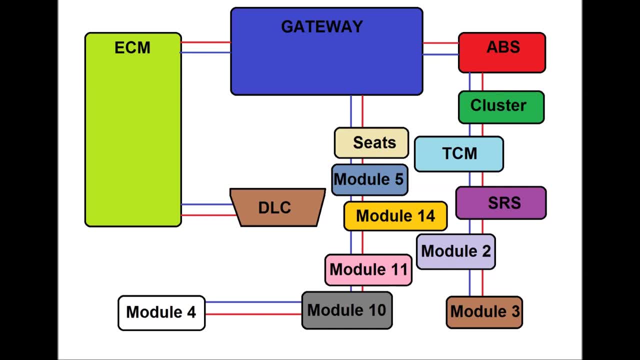 You have to find all these problems. basically, With what you've learned in this video, You can actually do that. It is possible for you to do that. It's gonna require, you know, some disassembly on your end trying to. You know see which you know. 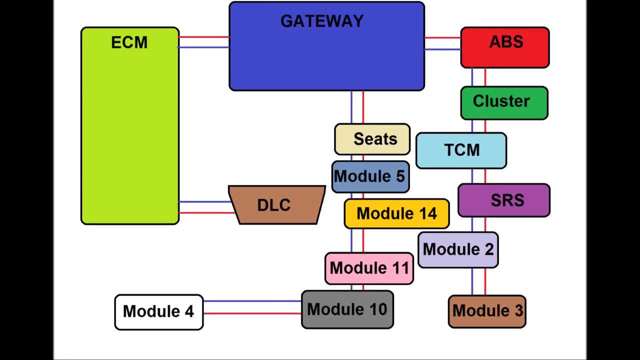 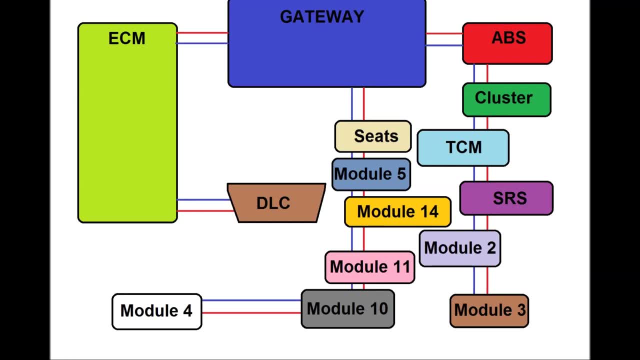 Where, where to find the gateway and what would it do? this, this and that, and oftentimes you know They. you do have a gateway module, which that does not restrict communication To the scanner. So again, it's a. there are variations of this, of what we're talking about in this video. 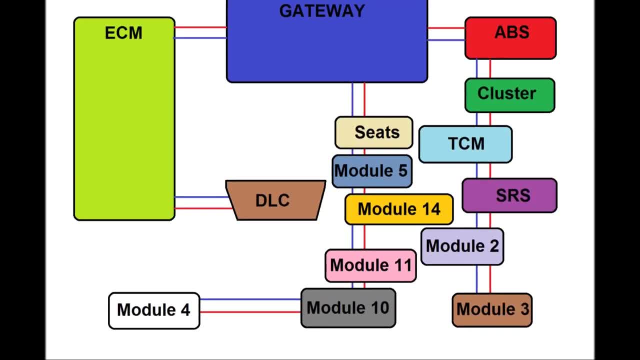 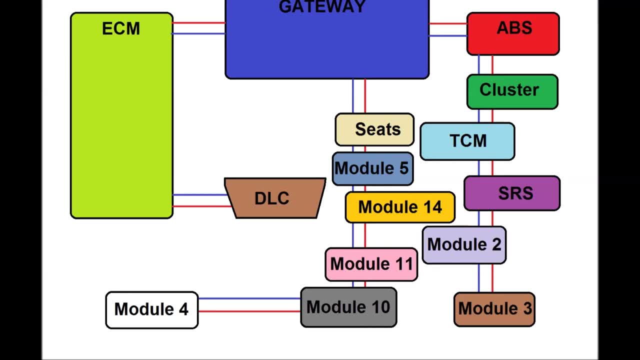 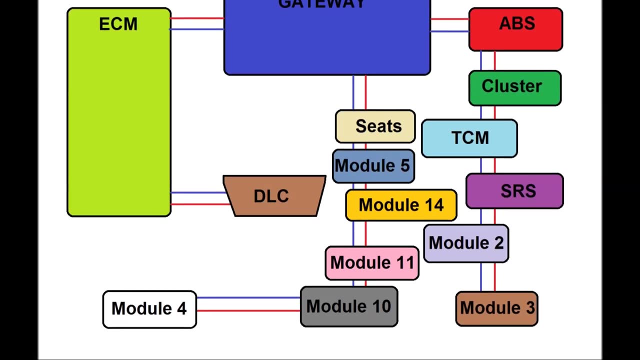 but the basic knowledge that you're gonna, that you're gaining right now with this video, is going to help you fix almost anything. a Problem that's related to the network, you know, to cant networks, you know, and again, you know we, You know, if you have the unit that we have, it's actually it's handy because it does a bunch of stuff. 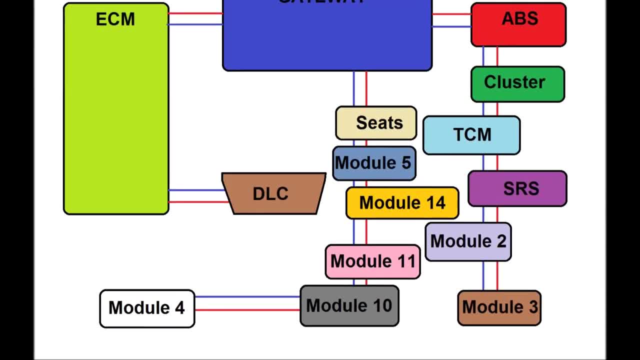 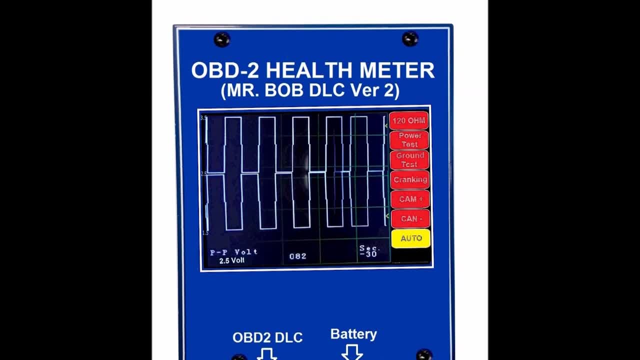 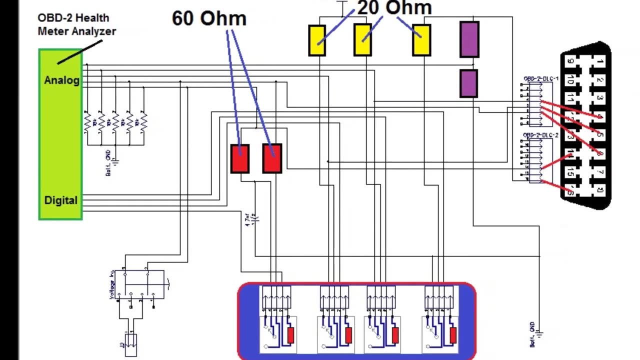 you know that, that usually you have to do it manually. it's not that you need our unit, but it's a good thing to have, and basically, that this is what we do in this video, so that you actually learn to analyze and pinpoint the certain factors, like resistance between the cables and this and that termination resistors. 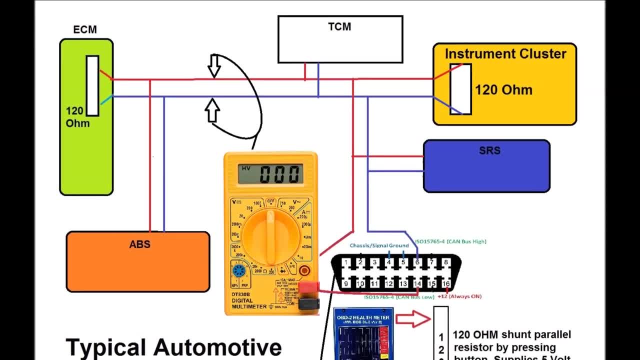 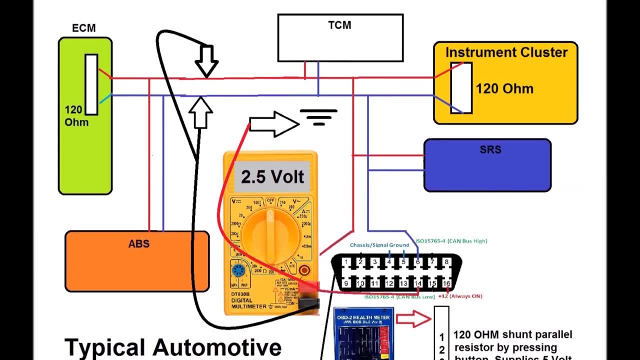 whether you have a gateway or not, how many networks do you have, how many modules, what's connected to what, and so on and so forth. Anyhow, we'd like to thank you for tuning into our channel, ADP Training. We suggest that you subscribe to our channel if you like it, or 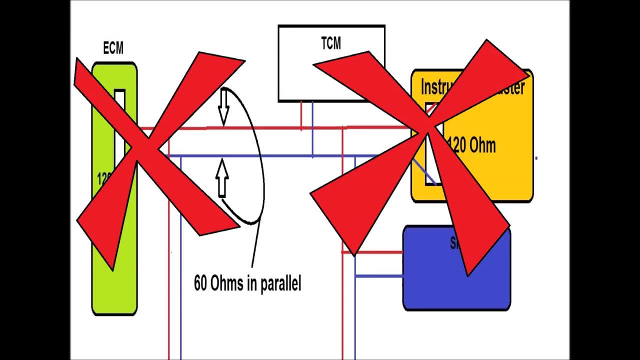 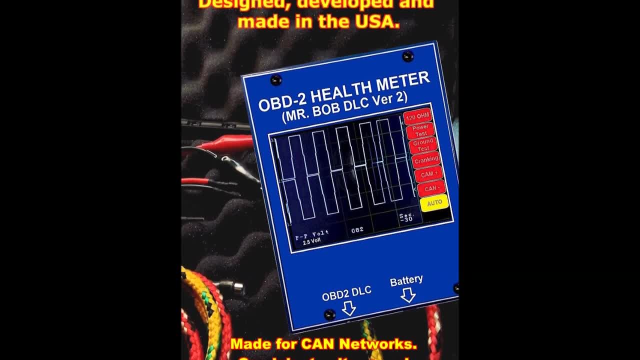 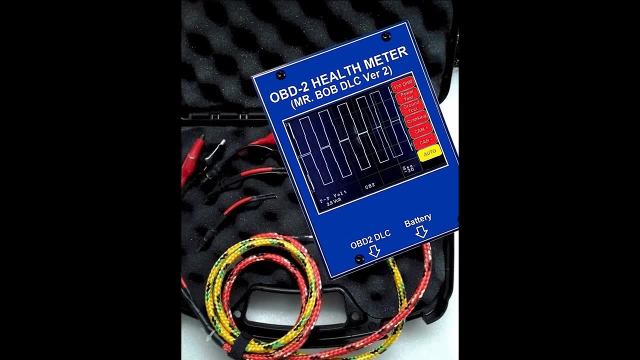 to our website Automotive Diagnostics and Publishing. It's actually autodiagnosticsandpublishingcom. You can find us on Facebook. You can find us on autodiagnosticsandpublishingcom. That's our Facebook page- or on Instagram. 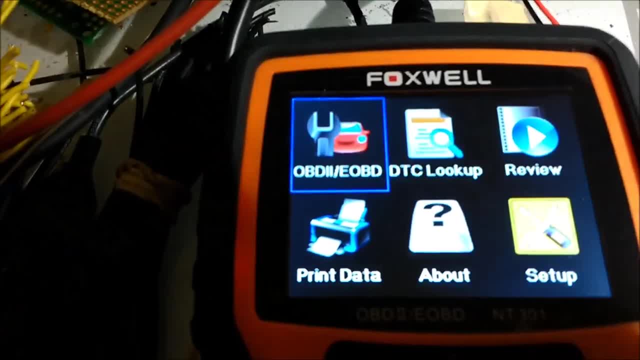 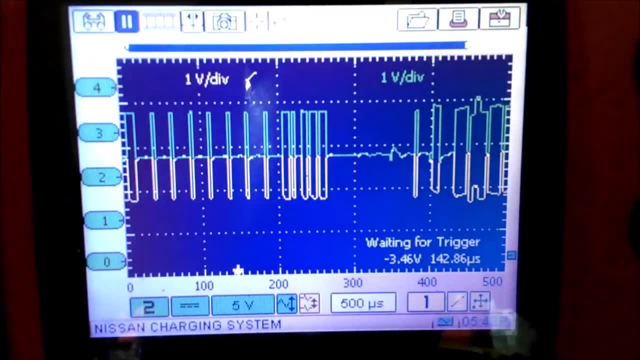 ADP Training. backslash or underscore YouTube, Which is ADP Training. It's our YouTube channel, okay, Which is basically, you know anything that's automotive On the high-end side. we go into the complicated issues, you know.